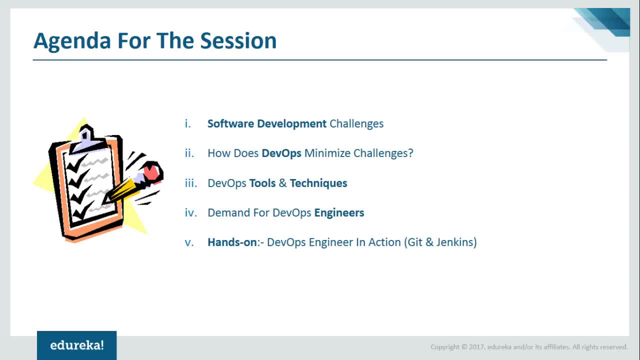 years are those of SDLC, agile development, scrum and, of course, now it's DevOps right. But what exactly is the need for DevOps right? DevOps is the most latest and by far the most the most efficient right. Why? Why is it that you know what caused DevOps to become? 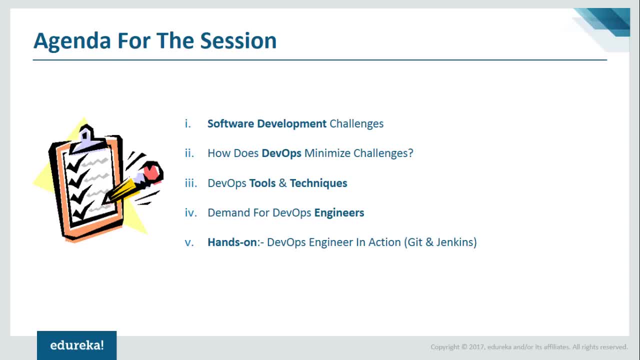 so popular? What is the need for DevOps? Let's look at that first. Okay, that'll be the first topic for today. We'll look at the different challenges with software development, Okay, and then I'll tell you how does DevOps minimize that challenge, And after that I will talk about. 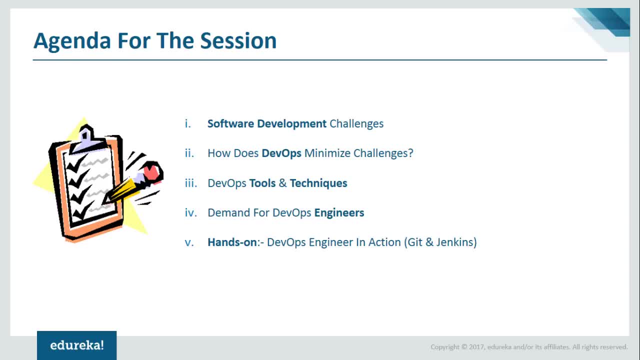 the DevOps tools and techniques which, of course, help us in enabling and achieving orchestration between the different DevOps tools. And that's actually the best part of DevOps: implementing the different tools, making a job easier, achieving automation- So that'll. 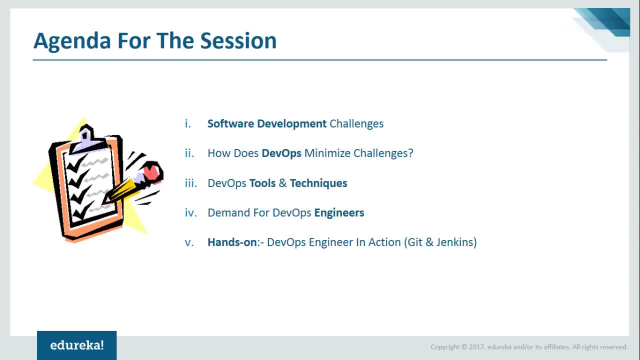 be another important topic That I'll talk about, And then, finally, I will talk about what is the demand for DevOps engineers, before finally giving you a hands on demonstration of a DevOps engineer in action. Okay, but this again is not going to be a very detailed demonstration, I'm just going. 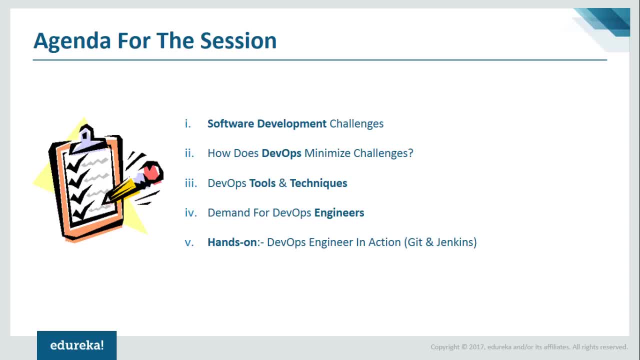 to use two tools in: Git and Jenkins. I'm going to show you a basic demonstration of how these two DevOps tools, which are the most popular DevOps tools out there, how they work and how easily we can benefit. Right, So that will be the agenda for today. So, without further. 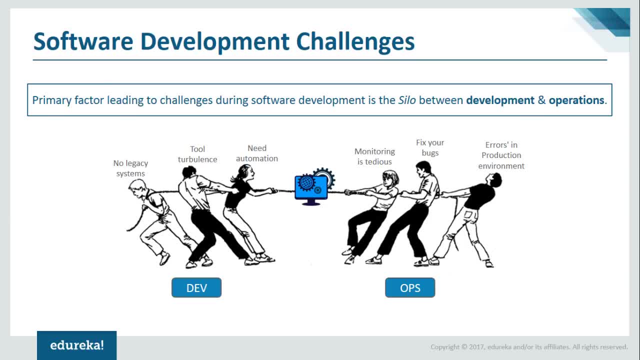 ado. without wasting much time, I'm going to start with my first topic, And that is the software development challenges. So the primary factor leading to challenges during software development is the silos that exists between the development team and the operations team. Okay, And as you can see from the image here, it's a very similar scenario out there. 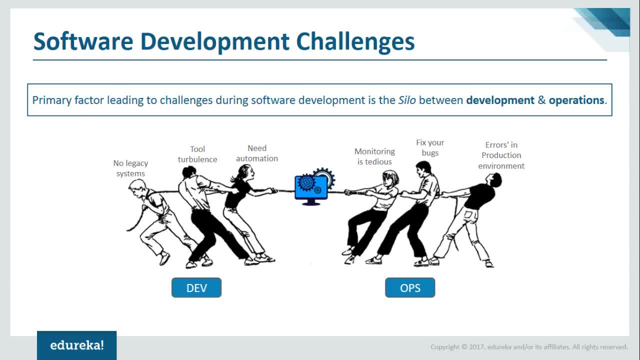 in the industry where you have the development team on one hand, on the and the operations team on the other hand, and they always have tussles. So they always get take blows at each other And they always have disagreements And they point fingers at each other whenever. 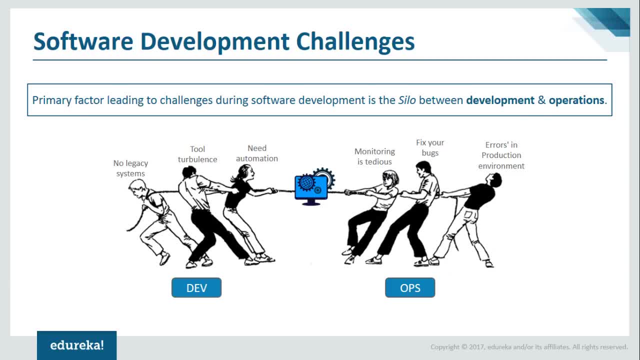 there is some kind of a mishap, that happens. Well, that's because the developers are responsible for just developing the code and testing the code and then giving it to the operations team, And then it's the operations teams responsibility to deploy that to the seeding server and then 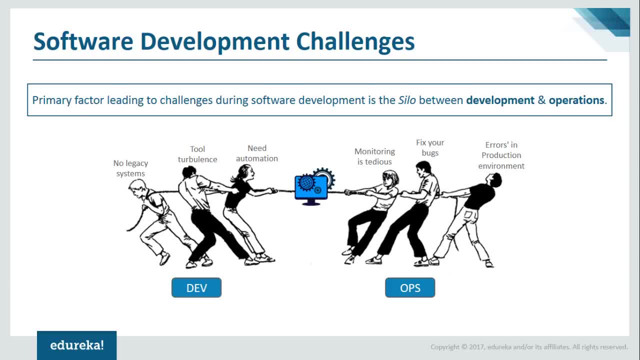 to the production server and then finally, you know, release it right and over here that the problem actually comes up. If there is any problem with respect to the code, you know whether there being a faulty bug in the code, then in that case the operations would start putting all the blame on the developers And 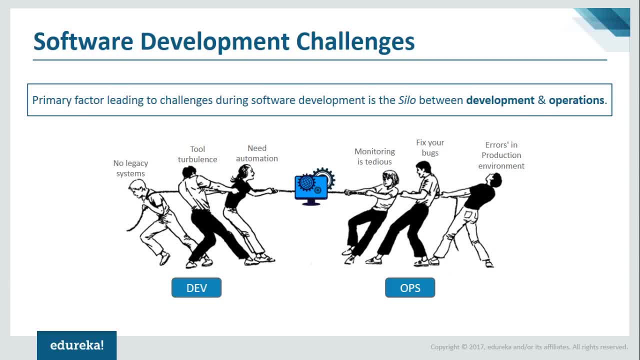 in fact, if there's a problem on the operations side, where if they're not able to deploy the code properly, then the developers would start blaming the operations there, So they would start saying that you don't have the system in place, you don't have the right. 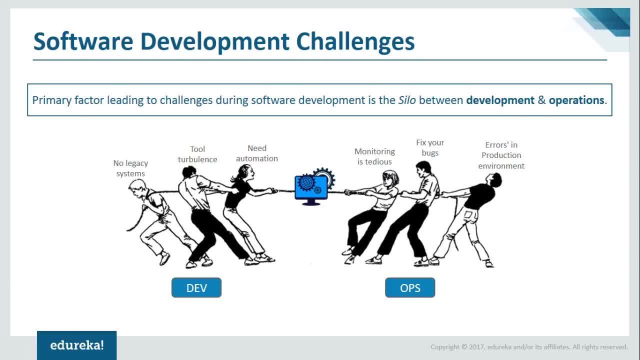 dependencies, you don't have the right tools and all these things. So it's a blame game that happens between the two And it's one thing which has been, which has, which has a bad effect on software development. So a lot of projects gets delayed And there is very 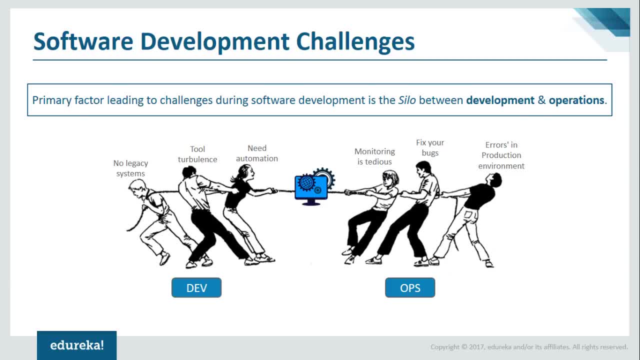 inefficient planning, and all these things happen Now. to eliminate this is what we have something called as DevOps. Okay, But before I go into more details about DevOps, let me talk about a few more challenges and problems that these people come up with. So, as you, 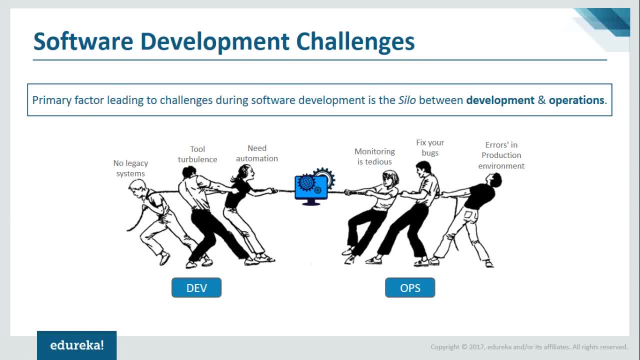 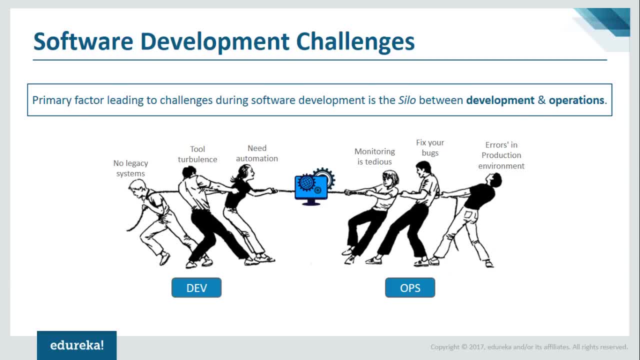 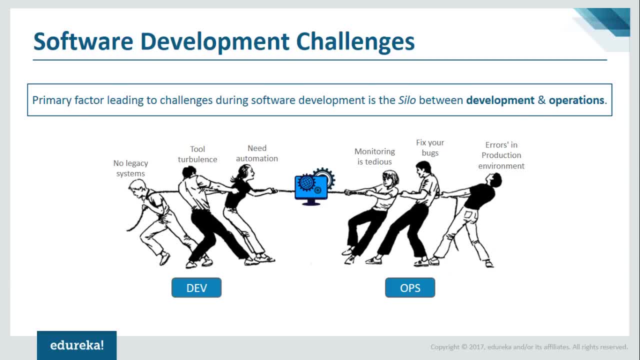 And that's where the operations would have a problem. So after the Playing is better everything. then they would know. the operations would complain that they cannot implement this stool and the developers would have a tussle and they will have to probably rebuild the software from scratch. 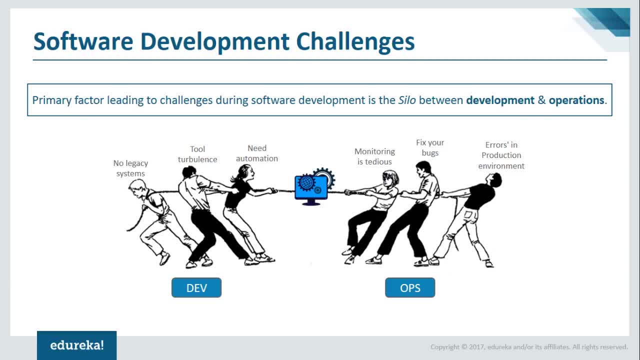 So that's one aspect of that's one aspect of the problem that they faced. Okay, developers most often complain that automation needs to be in place because a lot of automation helps in a big way. it reduces a lot of tasks. okay, being the technical guy, they are being the. 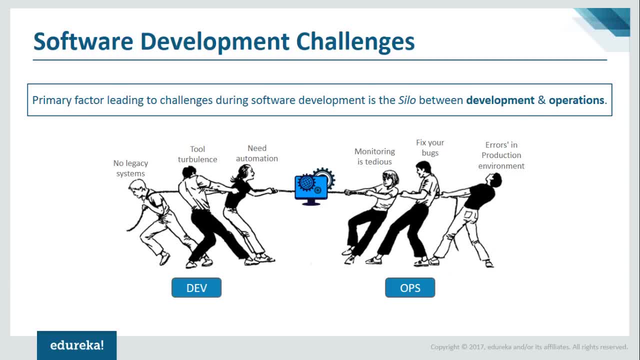 technical people. they know how to achieve it, but the operations would not always, you know, coordinate with the developers on that aspect. so that's one more complaint that the developers would have. now going to the operations people, those folks would start complaining that since the software or the 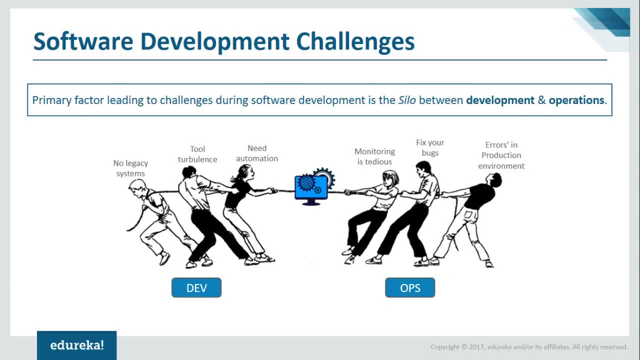 applications developed by someone else. them monitoring it on their own is little tedious, right? so that's one complaint that goes out. and they say that then there needs to be efficient monitoring, and even the developers have to be equally responsible for how the software is performing. if there is any bug in the code, then they should be able to fix that bug right away. 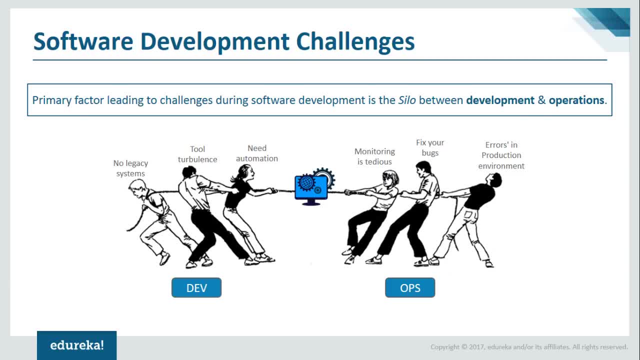 because if it's not fixed, then there is the onus is on the operations, right? so they are going to be held responsible. so they would be asked to fix that. and besides fixing bugs, there's no way to revert back the changes. so with operations, you know they. 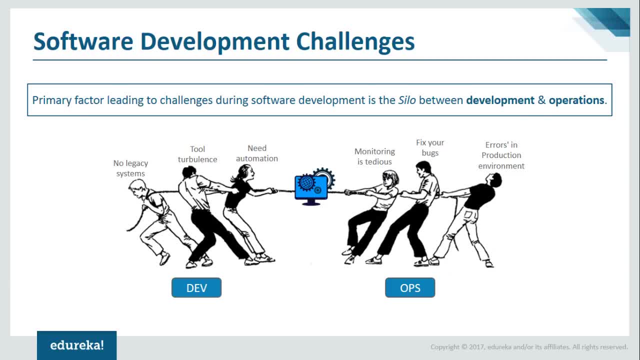 they are, their hands are tied in that place and, finally, the operations would also have problems in the production environment, like I told you earlier. so they would have different set of dependencies and libraries installed in their system and the developers would have developed the application based on the latest software. they would have updated to the beta latest dependencies. 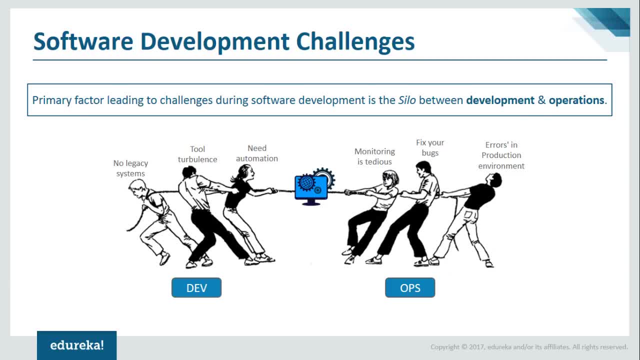 and that is something the operations would not have done, and that may be a reason why sometimes the application does not work well on the production. some features might not work even though it's working perfectly at the developers end. so developers would be complaining that it's your system that's. 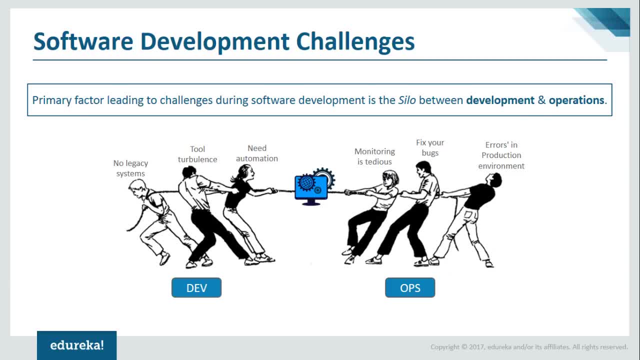 not that's causing the problem, and the operations would say that. no, that it's your code. so this is a very common analogy that comes with the software development challenges over the years and this is what has caused devops. okay, and, as you people know, the you people might be aware of the solution to this. 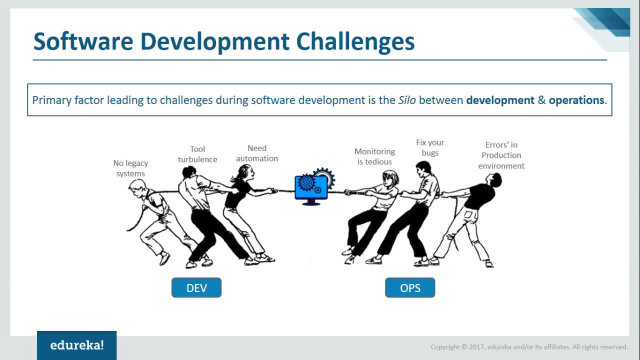 right now, right? so it's pretty simple. since the development of the software has been going on for a very long time and the there are two different teams here working separately to achieve a common task, they have this chance to blame each other, but if you merge them, you have the. 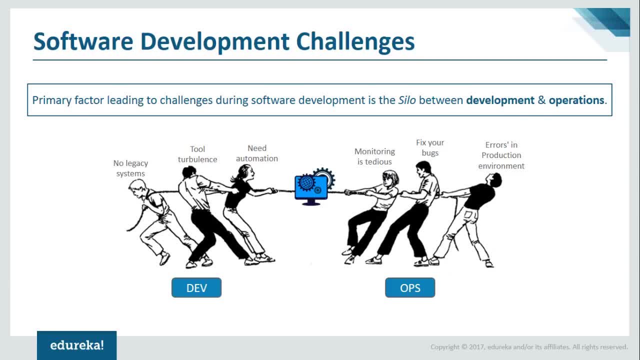 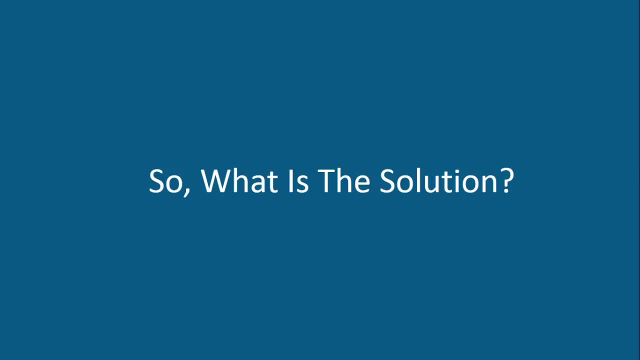 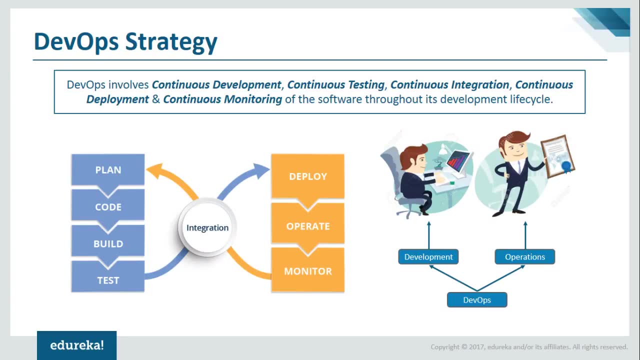 problems goes away, right, so dev and ops together- devops- solves all the problems, right, so that has to be the solution. I hope everyone here agrees with me. so on that note I'll go forward. and now let's see what is the devops strategy and what are the folks here that are working as devops- engineers? 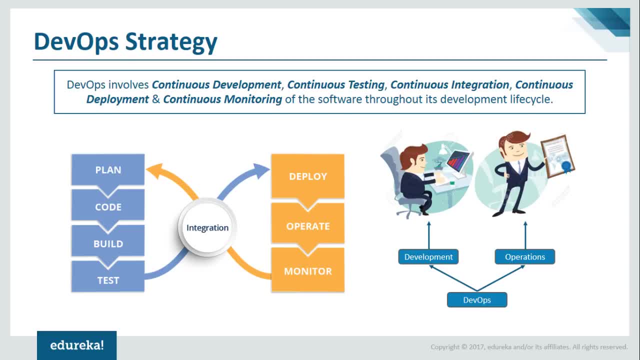 what is their responsibility? so devops engineers would not just, you know, be taking care of one aspect, they would not just be taking care of development, or they would not just be taking care of operations, they would have to take care of the entire lifecycle. okay, they have to be part of the planning, coding. 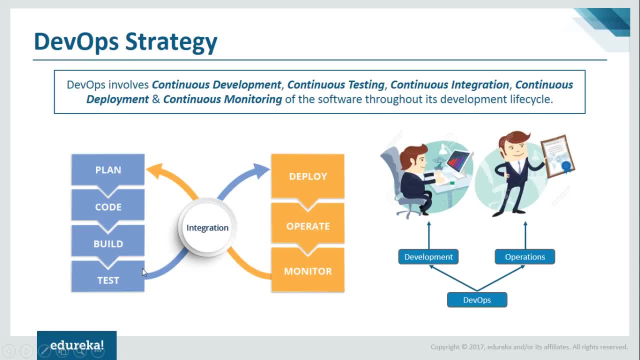 building that software, then testing it using different tools in they have to deploy to production, perform the operations on that and finally monitor how the application is performing. and finally, whenever there are changes, and with the next cycle, with the next release, they'll have to integrate those changes with the existing system. and 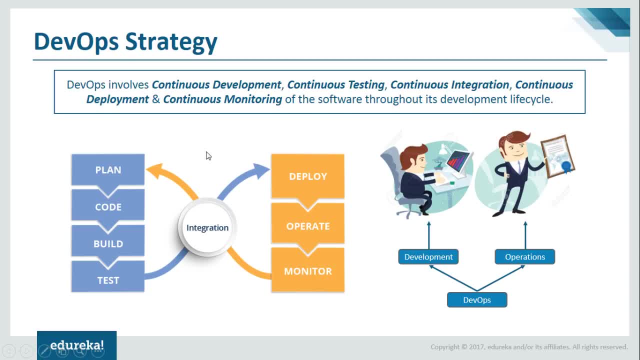 this is a never-ending cycle, so this is what devops engineers need to do. okay, and that is the same image that you can see here. so there's devops engineer that's working on a system that's probably coding, and then he is the same person. 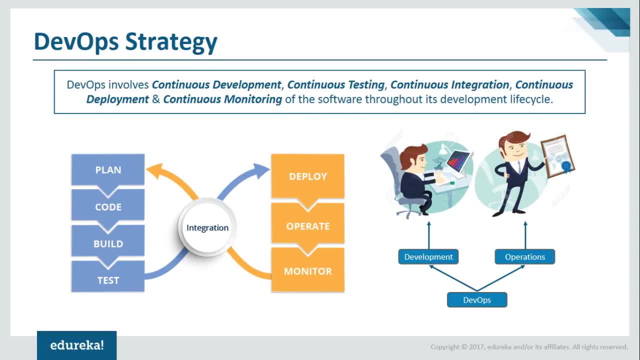 here he's also working on the operations aspect, so he's getting all the reports and all these things right. so the devops strategy, since it involves the engineers to have complete control of the application that's being developed, it involves continuous development, continuous testing, continuous integration, continuous development. 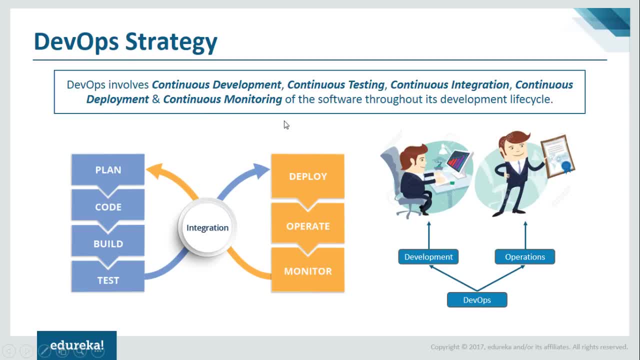 deployment and continuous monitoring of the software throughout its development lifecycle. right. so that's what the devops strategy preaches: that more responsibility needs to be taken. care needs to be taken up by these folks who are devops engineers, so the developers can't complain that it didn't work on. 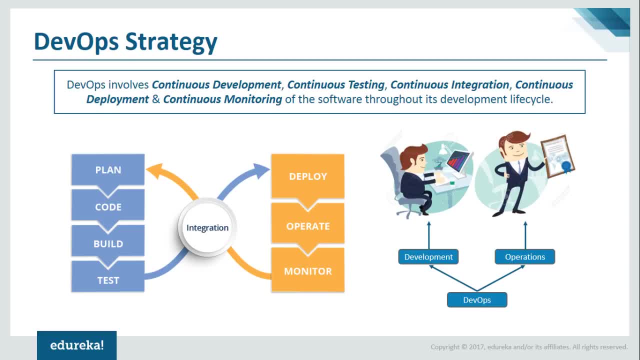 production, because they are now going to be responsible for that and since they are going to do it, so they will be able to immediately know where the bug is and why something's not working on production. and if something cannot be deployed to production, then what are the alternatives they can fix that. 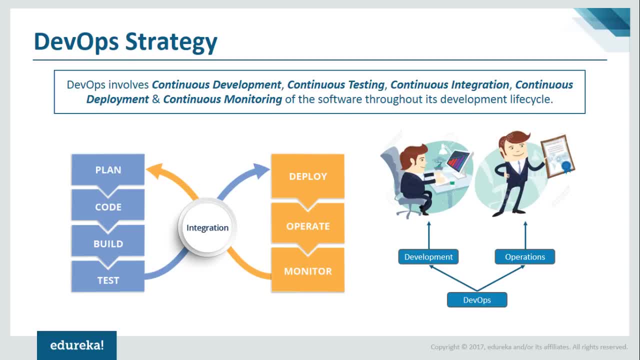 and with the help of devops, there's also scope for reverting back the changes right. we have version control systems which can be used to go back to the previous state and, you know, achieve a lot of automation and save a lot of time and benefit over the other. 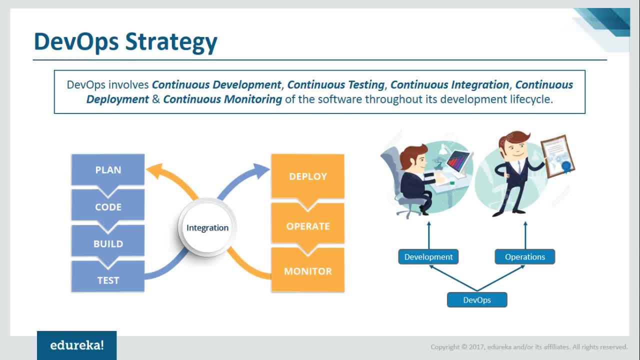 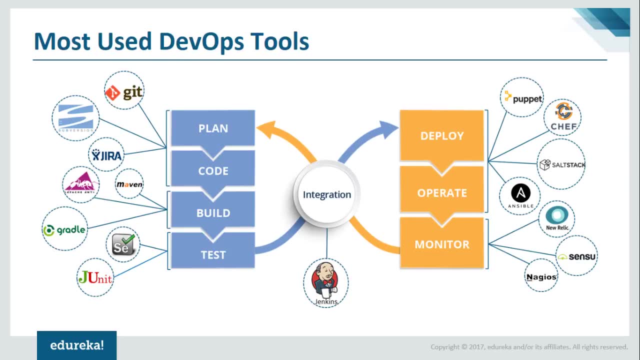 development methodologies. so now that we've spoken about the devops strategy and what the devops engineers are expected to do, let me go to the next slide and talk about some of the most popular and used devops tools. so these are the most moving tools in the market and we 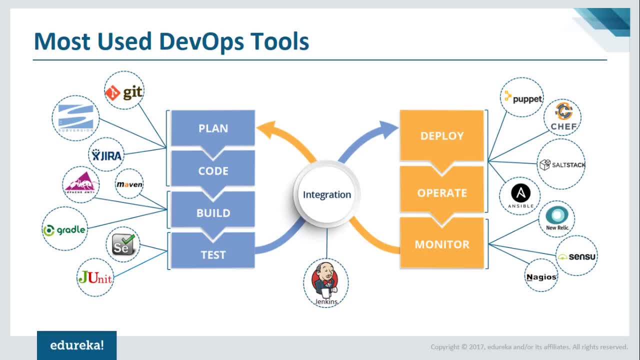 have different categories, so the same plan code: build, test, integration, deploy, operate and monitor. they are divided over various phases, so the plan and code. here we have three different tools in git: SVN and Jira. okay, this subversion is also called as SVN and these three tools are basically. 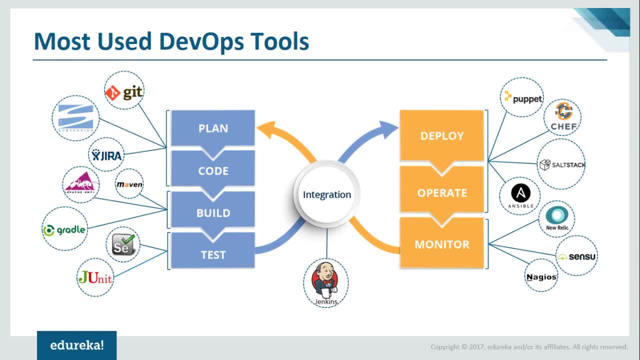 version control tools. okay, and they fall under this plan and code phase because, as as version control tools, what they do is they enable developers to write the code and build the code over here. okay, they can plan and they can code as per they wish to and they can make changes to it. 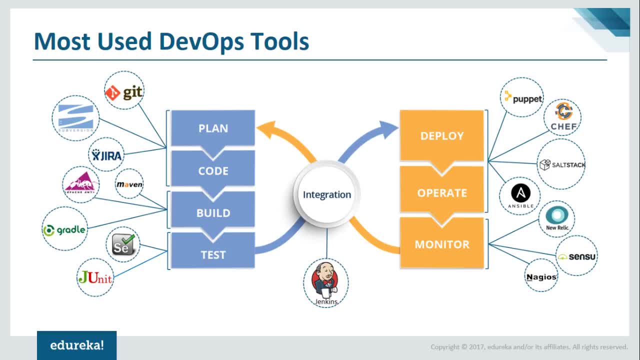 you know, act free will, so it's not like they have. they make. they write a set of code today and they make changes tomorrow, and you know they don't, they can't wrote back. so that's the thing with SVN. they don't have to worry about that, so even no matter. 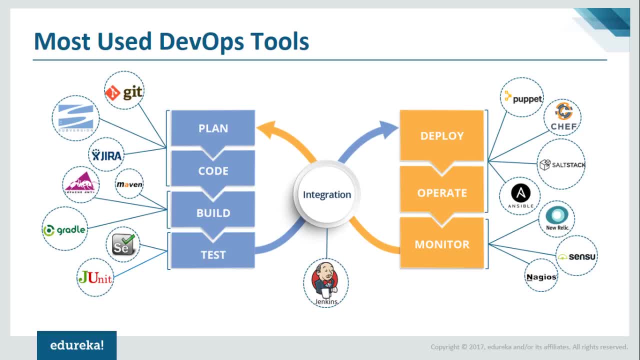 how many changes they make to the code, they can always revert back to a previous state because the version they would have committed to the SVN system or the git repository that would be tagged with a version. so if they are not happy with any version that they have released recently, or if 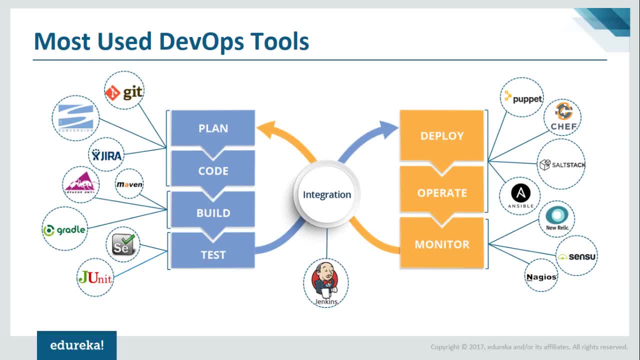 there's any bug over here, then they can always revert back to the previous state, which is, which was stable. so that's what these three tools can do, and that's what they do as continuous development tools, okay. and for building, we again have tools like maven and on. 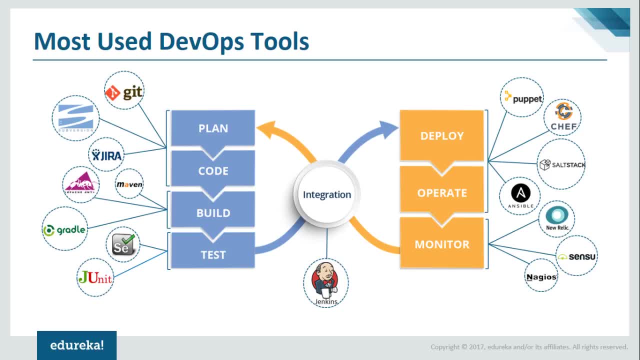 and Gradle. okay, now, these three tools are are for building and even they follow they come. they are actually part of the continuous testing phase. okay, they are used with the testing tools and the main responsibility for them is to use whatever code has been built right. so it would just package that and it would be ready to build for testing. so that's the. 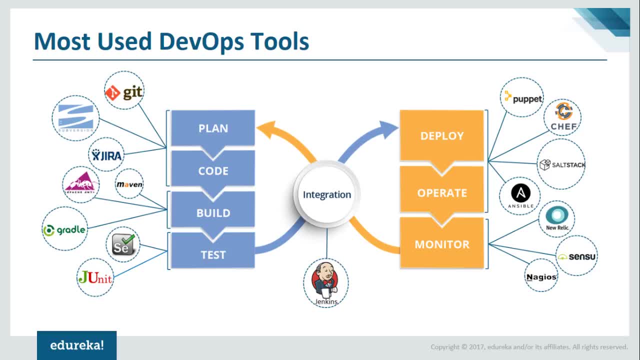 responsibility of these three tools and going on. the second part of the continuous testing phase involves these tools of selenium J unit and unit test energy. so these are the testing tools which would actually do the test. so this testing phase and the building phase, they together form the continuous testing phase, continuous testing part. right so in the continuous testing, 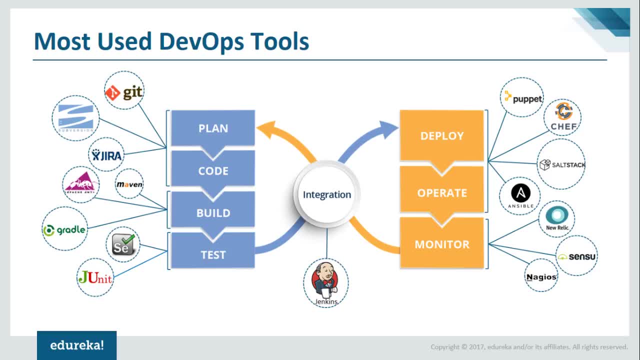 part. the code is built and it's tested. so the actual testing happens here and whenever there's, whenever the code is success or whenever it's a failure, then that can be worked upon, it can be improved, or it can also be integrated or it can be deployed. so this deployment happens with. 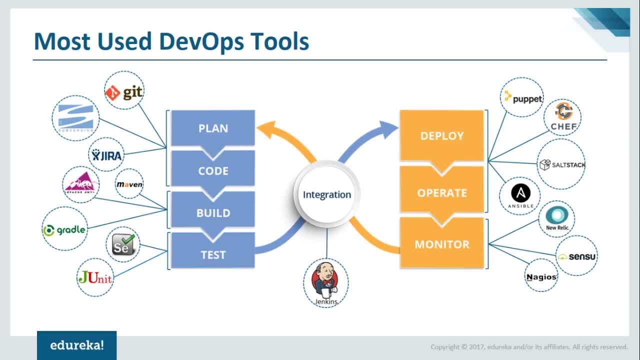 the help of uh in the, you know, for deployment, there is this phase of integration and uh, the integration that you see here- is one of the most important phases, and the tool that we use for integration is that of Jenkins. so Jenkins is probably my favorite tool because of what it can do and it is what 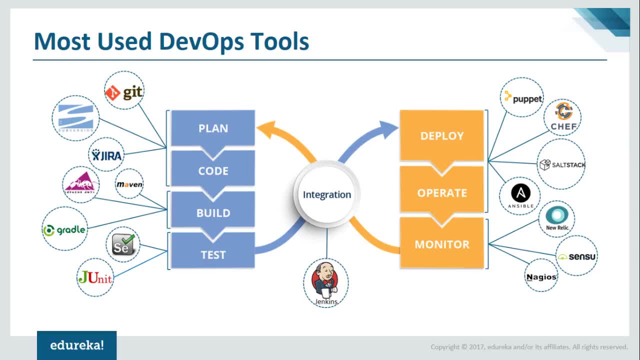 uh, encompasses the whole devops methodology. okay, so it's at the heart of the devops strategy, where it integrates everything. so if there is a new code that needs to be deployed, Jenkins can do that for you. if there is, uh, if your code suddenly stops working, then Jenkins will be there to notify. 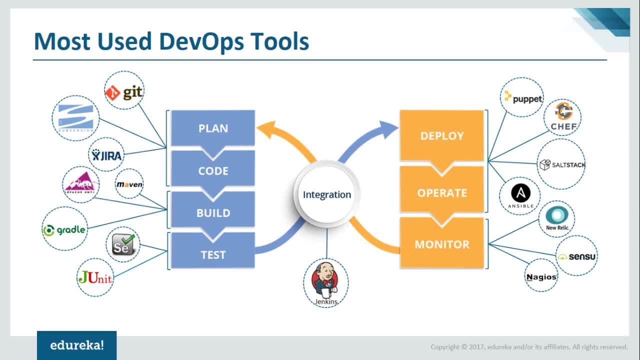 you of that problem and if you want to make changes to the existing code, then Jenkins can do that for you. it can do the integration, so it can do monitoring. so Jenkins is an all-in-one tool. it can do a lot of things with integrations and plugins to a number of tools here. 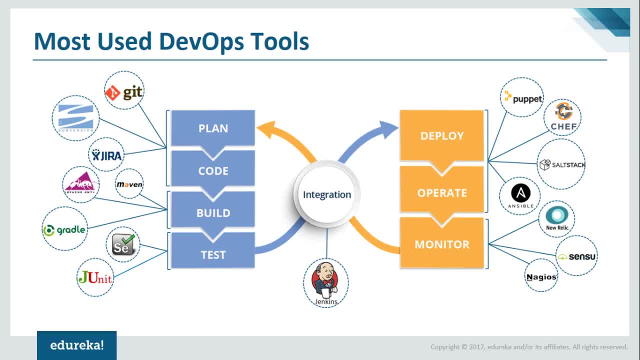 right. so and uh, Jenkins, its main uh integrations are with those of selenium, Maven, git and the configuration management tools and of course, uh, we're not talking about the Docker here. so Docker again is a really I know it's one of the best deployment tools which containerizes your 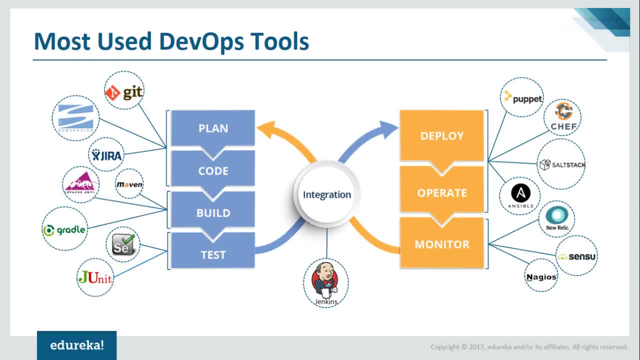 applications right. so that's what uh is the big benefit with Jenkins. so it can it. it basically blends in well with all the other tools, and then we have the deployment phase and the operation phase. so this forms the continuous, continuous deployment phase and over here, these four tools. 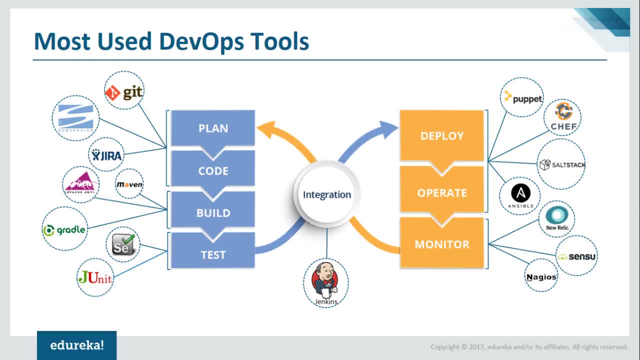 of puppet chef salt stack and ansible. they are the uh. they are the configuration management tools. okay, now, as configuration management tools, what they need to primarily do is to deploy all the code and uh, basically to deploy the code and the application to a number of servers, so on in the uh. so what happens in the industry is that you will have to 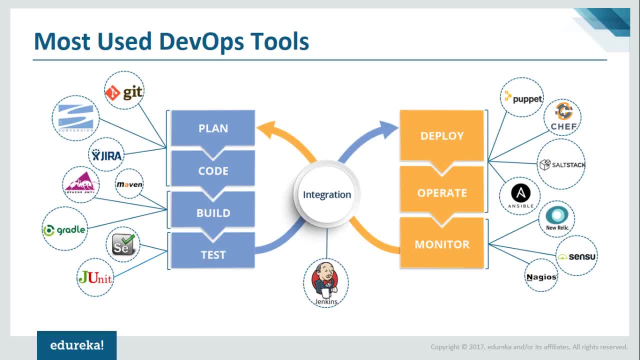 deploy your code or host your. if it's a web servers, you have to host it on multiple servers. right, you need to enable high, you need to have high availability and, uh, besides high availability, you it needs to be accessible by a lot of traffic, since there'll be a lot of load coming in. it needs. 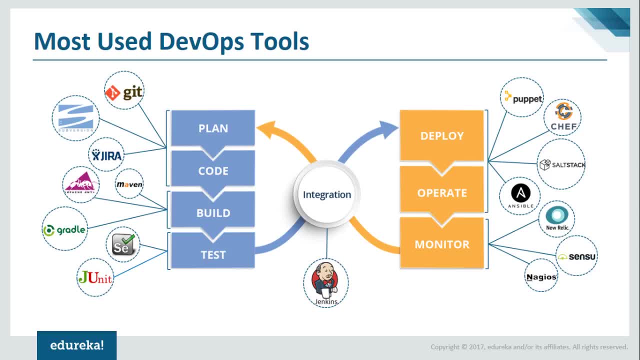 to be managed. so you'll need multiple servers and if it's fine, it's possible. if you're having to host just two or three servers, you can probably manually do it. but if you want to up to uh, 50 servers or 100 servers suddenly, so at that time you will have problems and even doing. 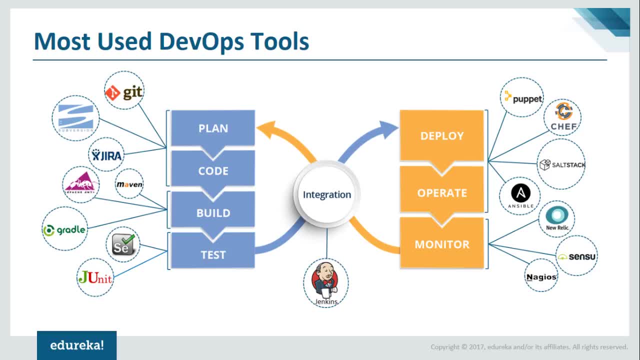 it once is fine, but if you want to make minor changes to the code that is deployed onto these servers, then it's a problem, right? so that's where these configuration management tools come in. so with these tools, you can easily deploy these code changes and deploy the code itself from scratch. 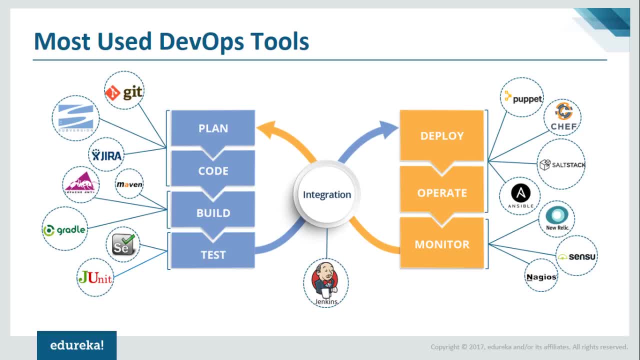 on any number of servers. so they are. basically, they work on the basis of master slave architecture where, with the help of master, we can deploy the code from scratch and deploy the code from scratch to multiple slaves, and each of these slaves would be the different servers. so that's what the 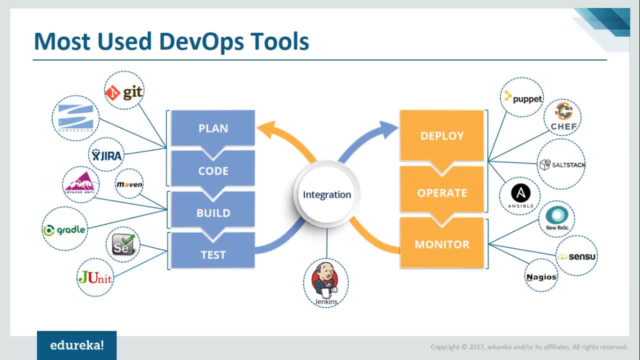 continuous deployment phase, comprises of it, comprises of it holds the deployment and the operation as a part of it. and finally, here comes the monitoring phase. it may be the last, but certainly not the least, because it is the monitoring phase which tells if your application is working perfectly, if, if it's all fine, if there's any downtime, if something fails, if something. 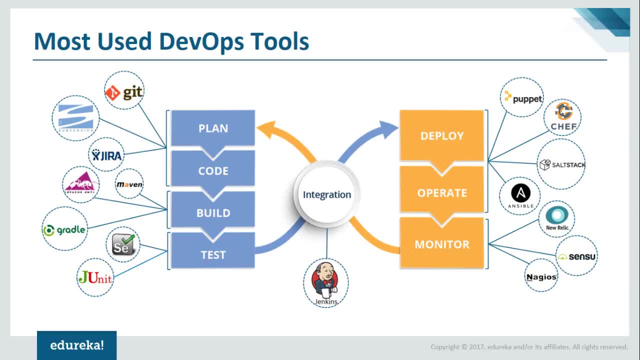 happens if your system is not working. all these errors would be. uh, you know, you would know only with the help of monitoring right. so you have to always have a look at how your application is performing, and the tools for that are those of new relic, sensu and nagios. so these are some. 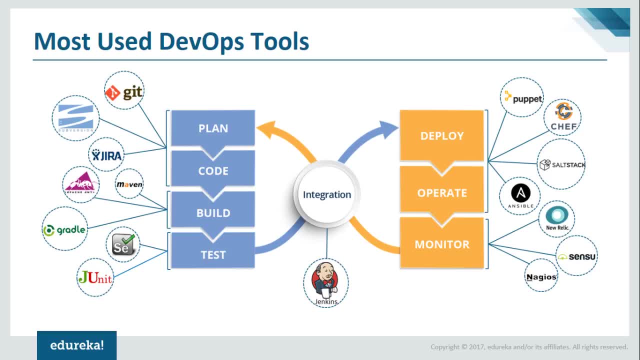 of the most popular tools and uh, yeah, that's how they work together. they work in tandem, right? so any doubts, guys, uh do drop in. if you have any doubts, uh do let me know. at this point, guys, so i'll just give you people a couple of minutes to put in your questions. 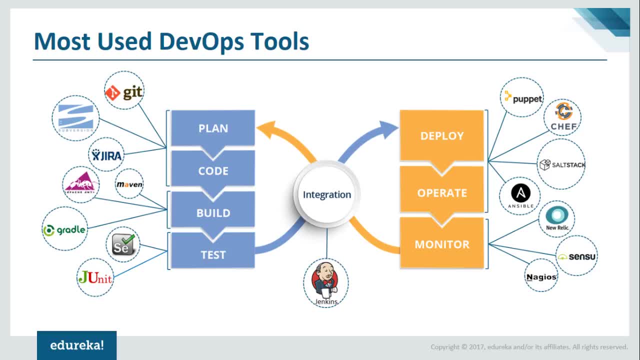 okay. so i'm just going to mute myself till then. okay. so there's an interesting question here from bupati. he's asking: in the future, would there be no jobs for test engineers? well, it's not like that. so you would, uh, definitely have, you would. 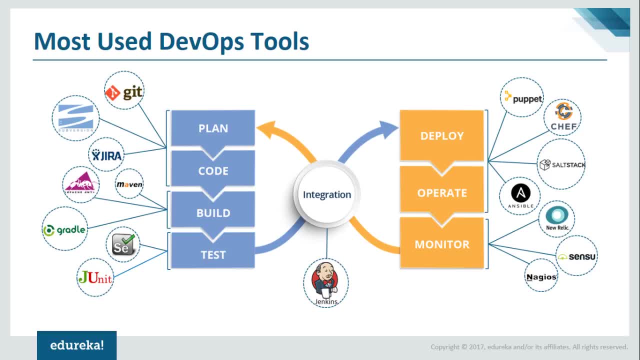 definitely have openings for test engineers. they are also a part of this devops life cycle. okay, so the devops engineers would also be doing that part and it would not be just a different phases. like i said, devops comprises of a lot of things and they would all be working together. so you 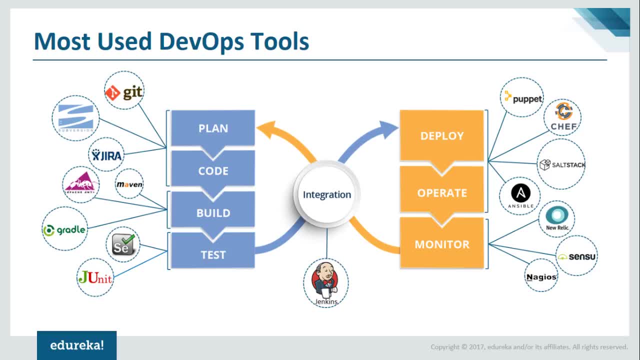 will have to have multiple skill sets. so gone are the days that you can just sit on one particular fruit and enjoy the taste, so you'll have to have multiple skills. so that's how this happens, okay, so guys, uh, anyways, let me get back to my uh session here. okay, let me continue with my uh session. 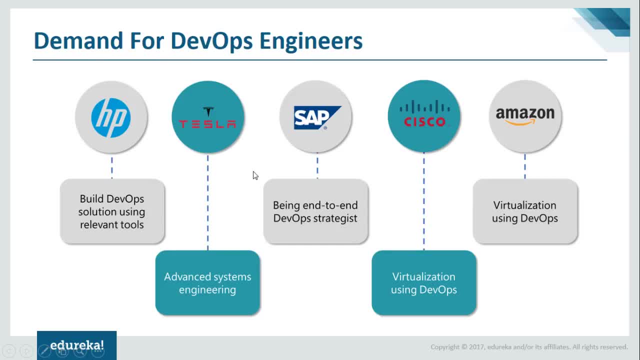 so i'll take up more questions later on. so, yeah, there's just one more slide here before i go to my demonstration, and that is: uh, what is the demand for devops engineers? okay, you guys might have by now realized how uh devops is the future. so there is some. 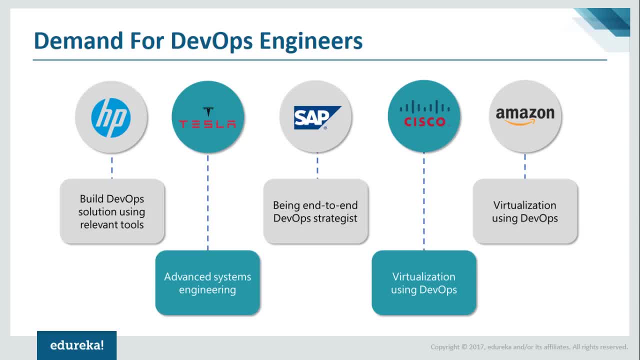 more proof here and, as you can see, some of the top companies over here in HP, Tesla, sap, Cisco and Amazon, they're all hiring devops and uh, it is these devops, engineers, whom they are rapidly looking to. you know groom and uh hire. so if you look at HP, they are. they say that they want to. 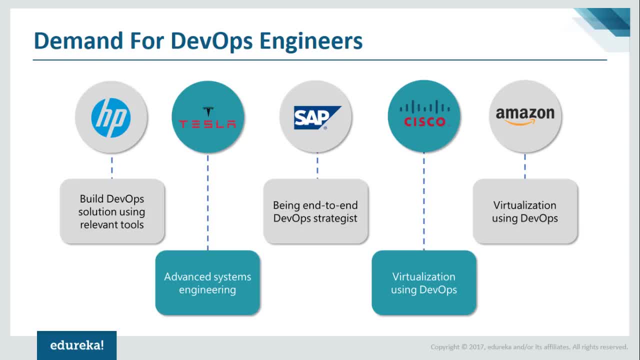 build devops solution using relevant tools, because, of course, they are a big MNC, right, so they have various services and, uh, absolutely it makes sense when they say that they want to make use of multiple devops tools, and it's the engineers who would be doing that for them. 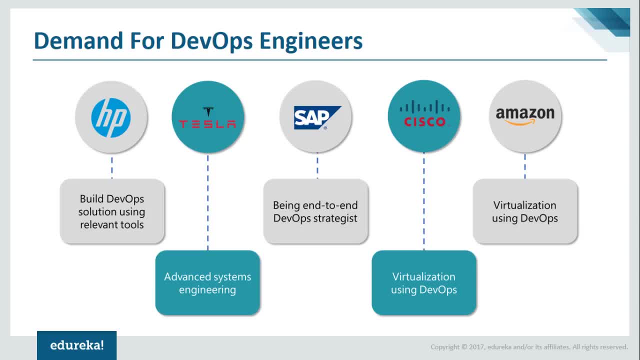 and Tesla for advanced system engineering, sap for end-to-end devops strategist. well, this is another interesting thing, because there is just so much to do with devops and it's an unexplored field. it's still young and there's so much that you can do as a devops strategist. and, uh yeah, sap are just. 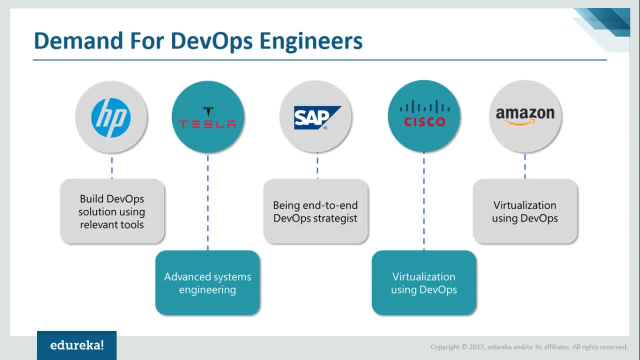 doing that and, uh, this shows that you know how much how important these devops engineers would be for them. and the same thing with Cisco and Amazon. they are trying to implement virtualization using devops. so this is just on a. I've just given you a basic uh idea of how the demand for them is. so I've not 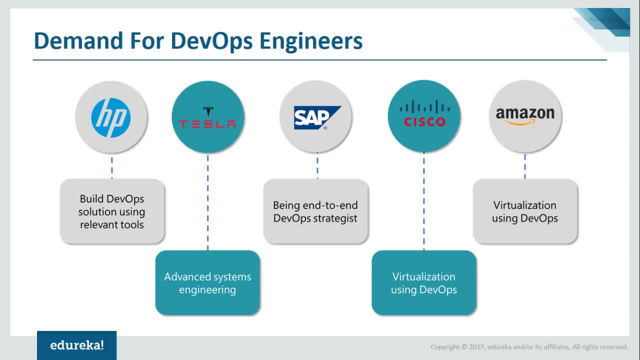 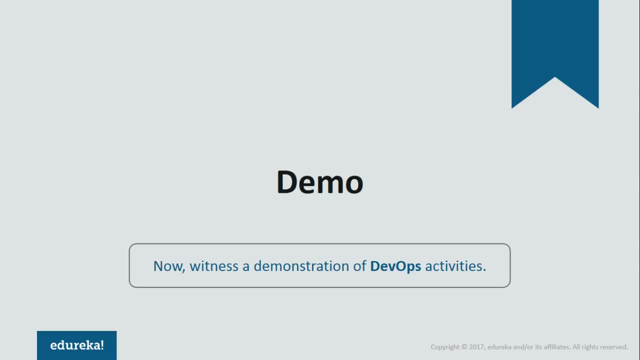 even included all the software service companies here. I have not included any of these startups, it's just some of the top companies. so to just give you an idea of, uh, you know how the demand is, so, uh, well, in the meanwhile, uh, I can go to my demonstration because, uh, that's the end of my 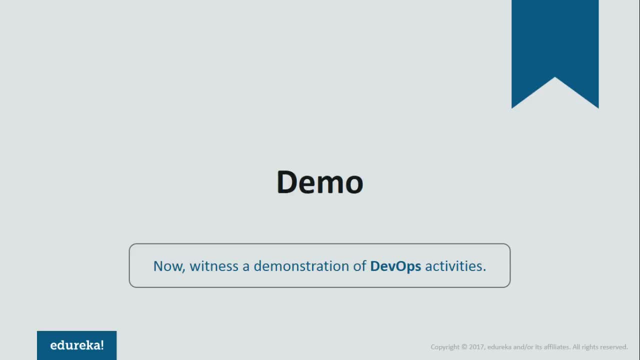 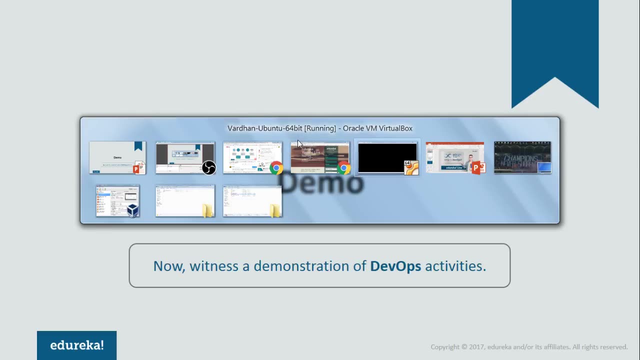 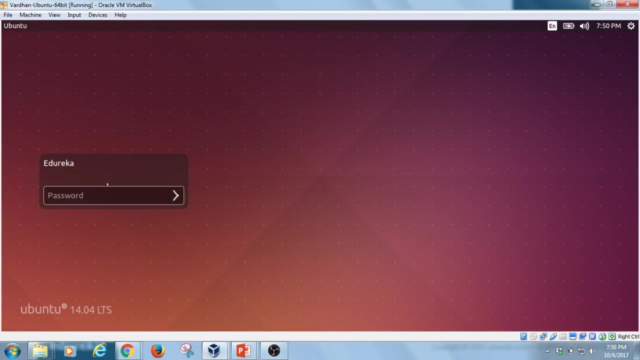 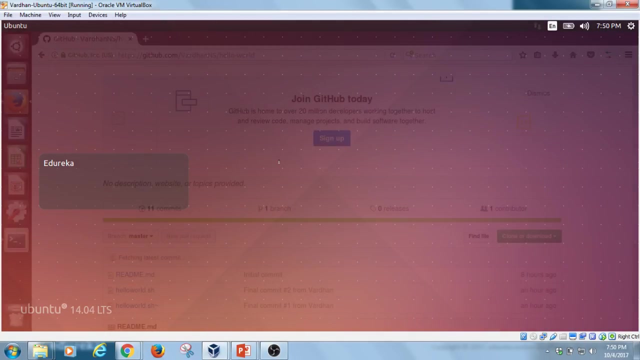 uh, slides and uh, to go to my demonstration. what I need to do first is I need to open my virtual machine, right? so, guys, uh, do give me a confirmation. if you can see my virtual machine, can you see it, guys? okay, all right, so please bear with me. 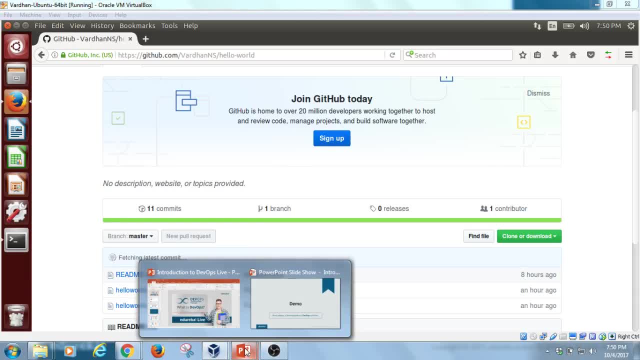 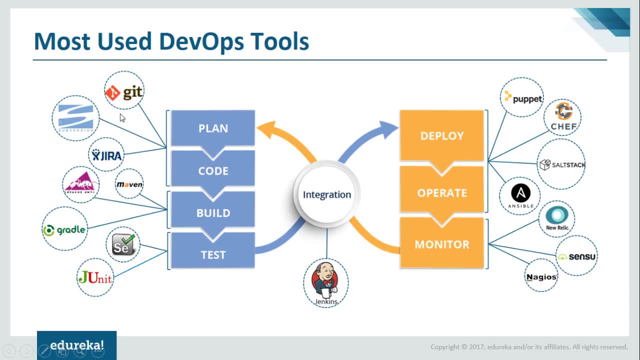 my VM is a little slow, but uh, anyways. uh, the demo that I'm gonna show you is basically using the two tools of git and Jenkins. okay, like I told you, git is going to be used for storing my code and pulling the code to basically be stored as a central repository for my code, right, and my Jenkins. 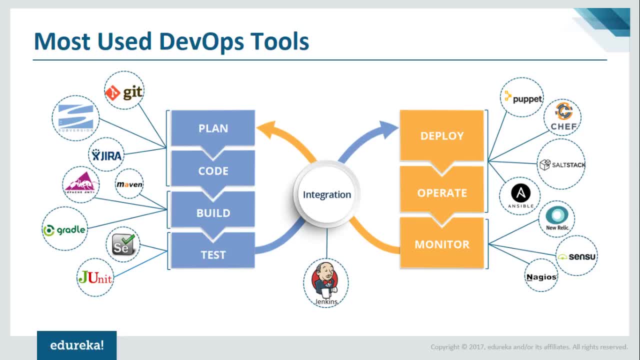 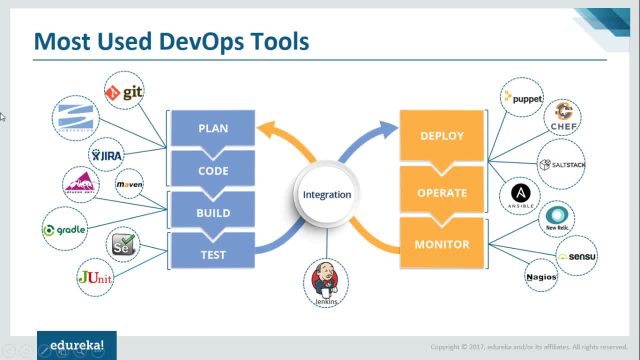 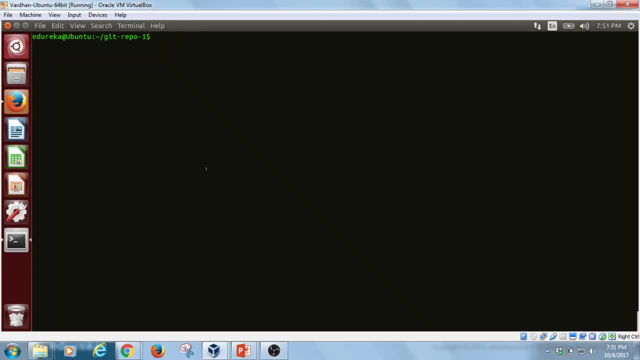 is there and get. okay, so let me just show that implementation on my system. so this is my VM, this is my terminal. okay, so I'm here. let me just see you to the git repository. so here you can see that there is one hello world file and then there's a readme file. so there's readme file. 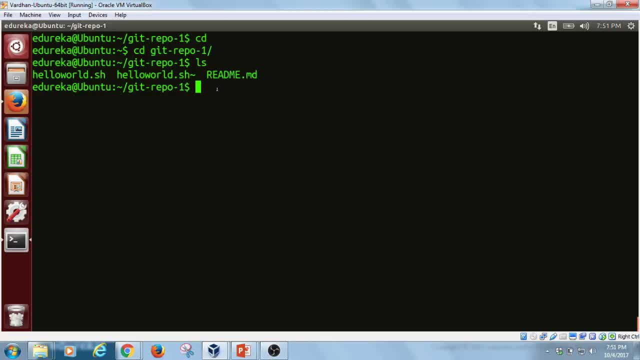 comes with your git repository. so if you initiate any repository in git or readme, file comes with it and my hello world file here. let me just do a cat and show you what is there here. so it's a simple batch file which I have created which says hecko, hello world and hecko hi from Edureka. okay, 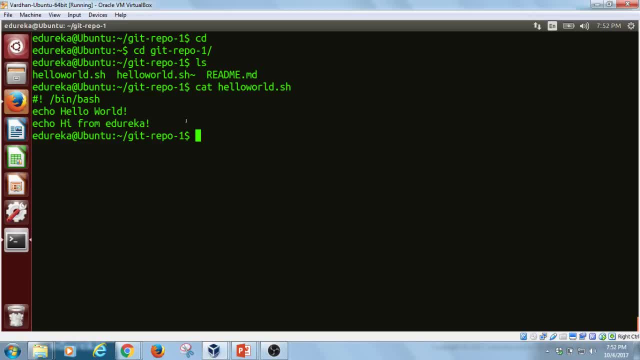 now it's a very basic demonstration and I'm not going to go into details of how the code is, you know, being managed over here and how it's going to be deployed. I've done that in some of my previous sessions, where I've showed you how to deploy an angular application, how to deploy a main stack. 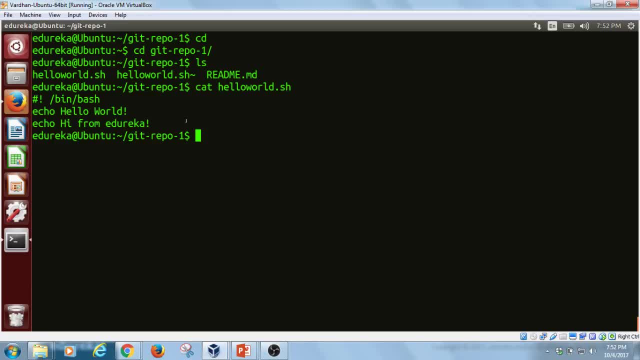 application and all those things. so this is a basic session where here I'm just going to show you how git and Jenkins can be used together. okay, and git being very popular and one of the most important or the fundamental tool for code development, I'm going to show you how that happens. 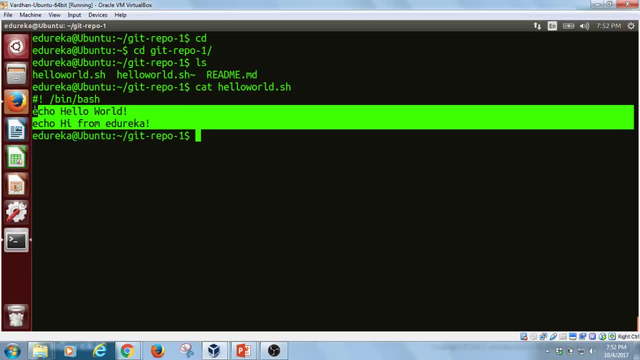 so this is what is there in my batch file and if I execute it from my terminal, this is the output that you get right? so even when I run my well, what I did here is: I did, I did cat hello world. so if I, if I want to execute this batch file, I do a bash. 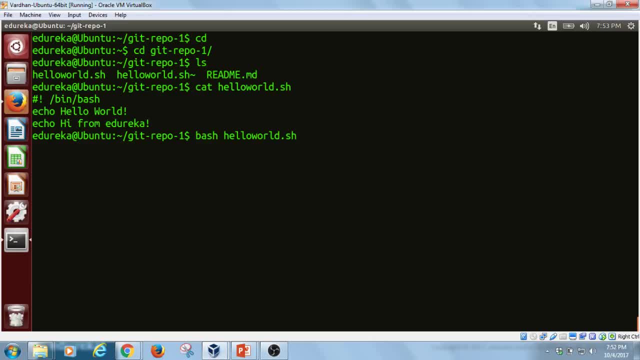 and hello world dot sh. right, and for those people who don't know what bash is, bash is basically to execute. this is used to execute any, any shell, any batch file, okay, and inside the batch file, commands would be specified and whatever is specified, that would be straight away executed. so if you see here, 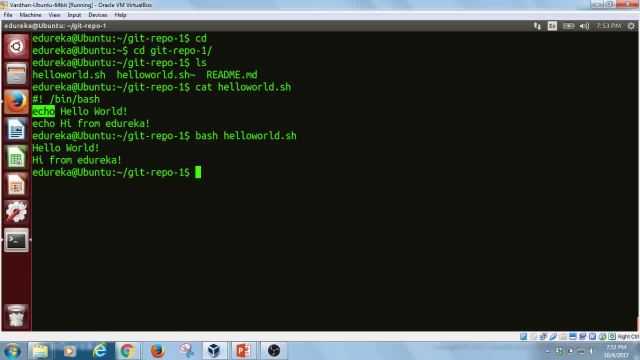 I've said echo hello world and echo hi from edureka. okay, now when I did batch, hello world dot sh, these two commands were simply executed. okay, the echo command simply executed hello world and in the second line, the echo command simply executed hi from edureka. so that's what a batch file does. 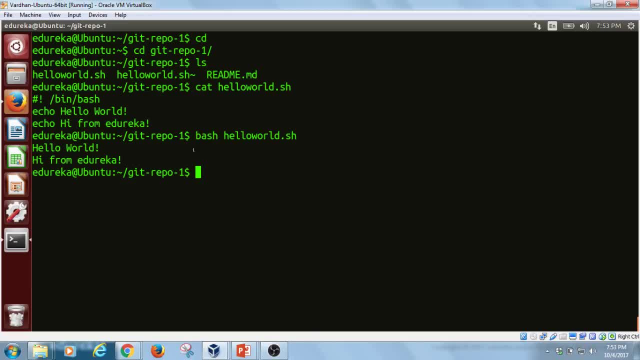 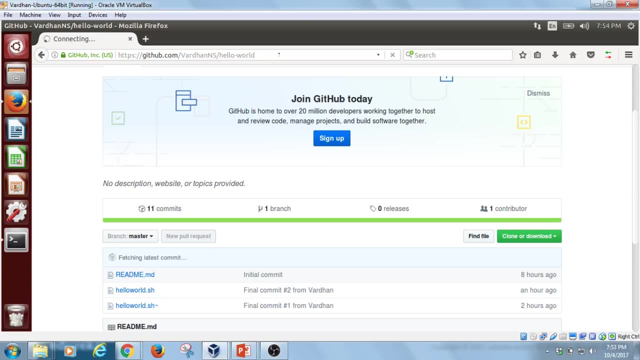 uh, sorry, a bash file does okay, and uh, executing this through Jenkins is what I'm going to show you. but before I show any execution over there, let me first show my GitHub repository. okay, so, using my Jenkins, I'm gonna pull this code from my GitHub repository. so, as you people are aware, uh, this, 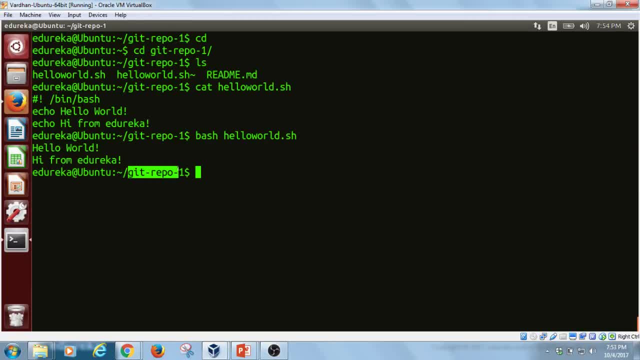 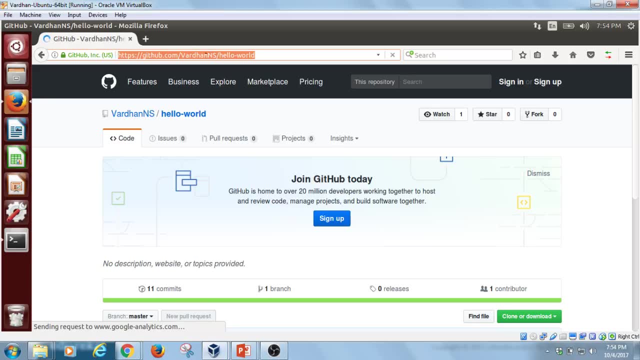 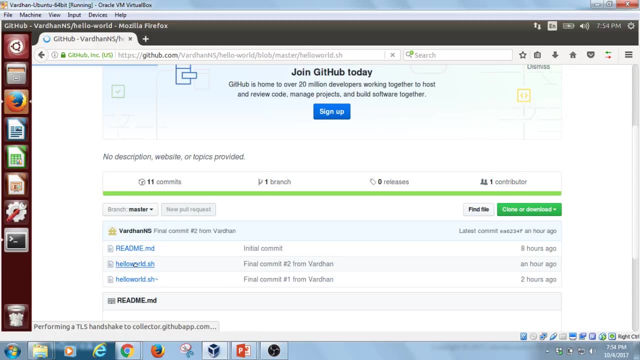 repository of mine: slash home. slash edureka. slash git repo one. this is a git repository and this is linked to my URL at this one: githubcom. slash var than ns. slash hello world. okay, so we have the same code over here, the hello world dot sh, and, as you can see, we have the same two lines: echo- hello world. 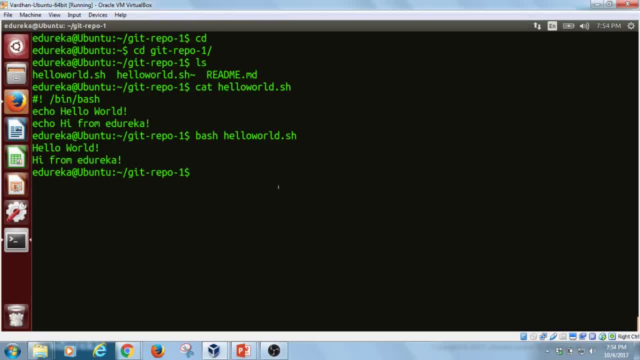 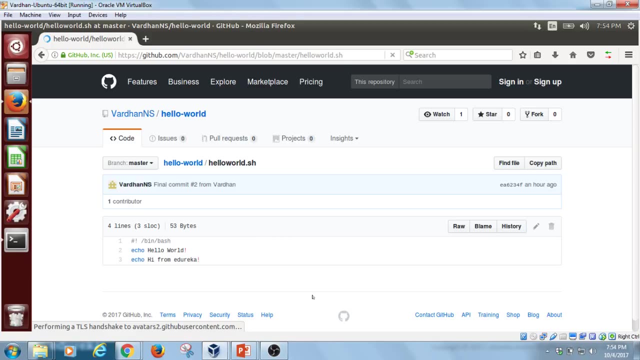 and echo. hi from edureka. now, uh, I want to show you how git works. okay, before I show you something with the Jenkins, I want to make changes to this code and show you how I can push code using git. and when I push code from git, those changes would be also tracked in my GitHub repository. 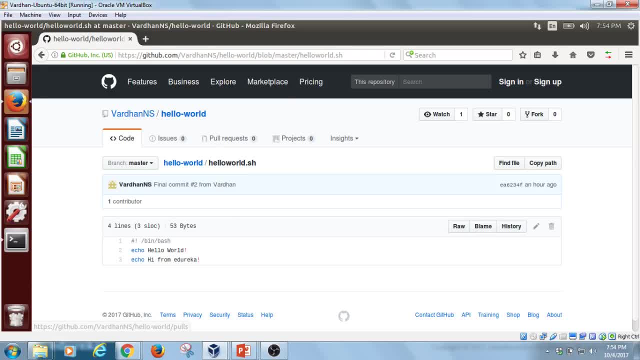 okay, and from the GitHub repository, I can use Jenkins to execute this code. so what happens in the industry is, whenever such code is, uh, you know- being developed, it'll be developed by a lot of people right at the same time, so you will have, uh, say, five to six developers. 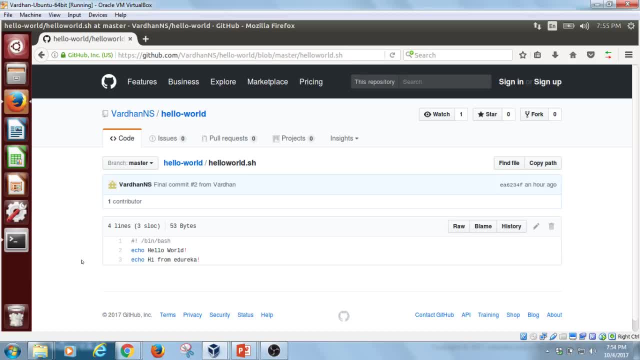 working on the code and they will all be making changes and developing their own code. and as and when they make changes and as when they develop a couple of lines of code, they will be pushing it to GitHub and from GitHub, the final code will be: would be sent to deployment. it would first be tested and 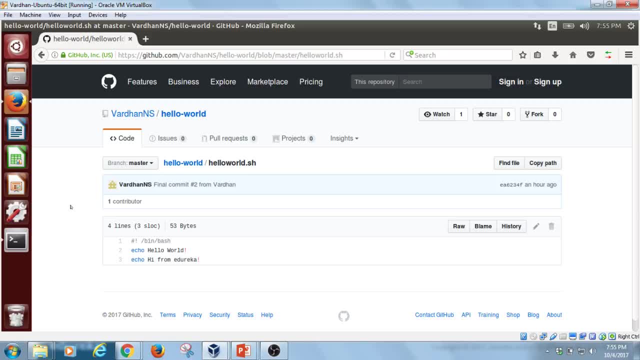 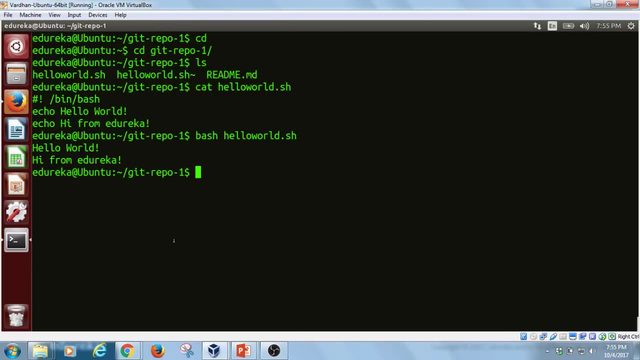 the staging server and then it would be released to production. so, basically, GitHub is used as the resource from where the code is managed centrally. and uh, yeah, we can. people can connect to GitHub from their local systems itself. so, as a developer, look at me in action. see what kind of changes I 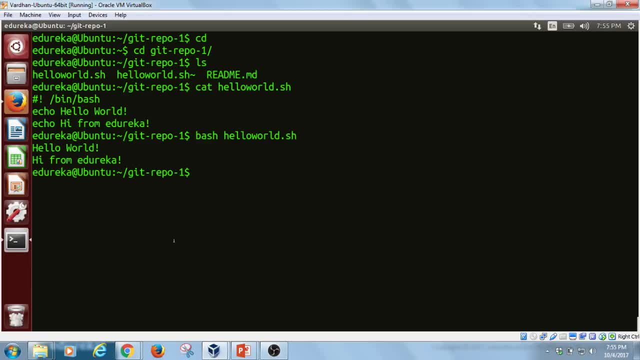 make to my GitHub repository and how I push my changes to the GitHub, and then I'll show you how that can be executed through Jenkins. okay, so first of all, if I want to edit this file, let me do a pseudo gedit: hello world dot sh. okay, and this is the password. 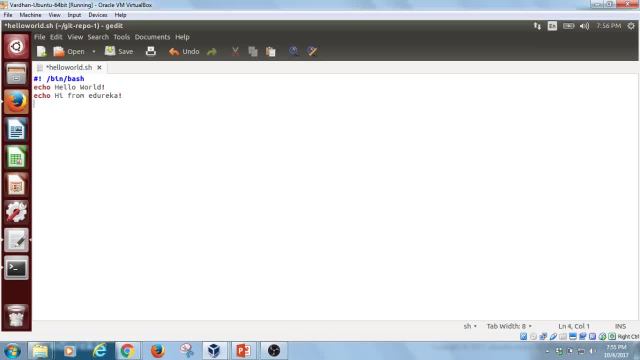 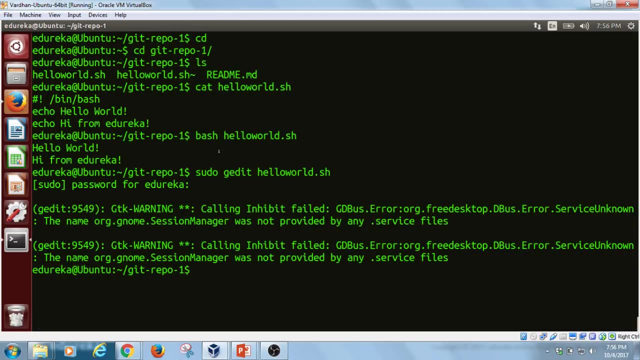 okay, so I don't want to make major changes. so let me just uh say, let me enter another echo command and say, um, your instructor is vardhan. okay, I'm gonna save this. so there's an extra line that I've added here. so, even if it's with respect to any Python or Java application, any kind of 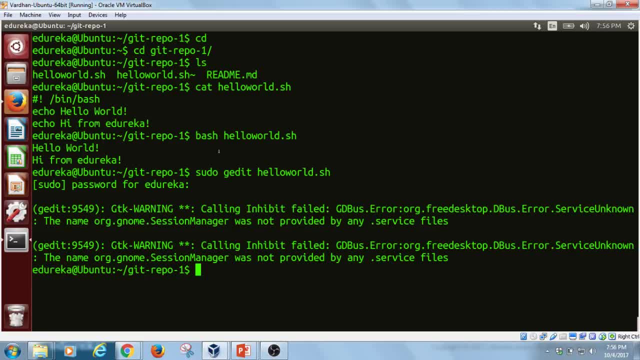 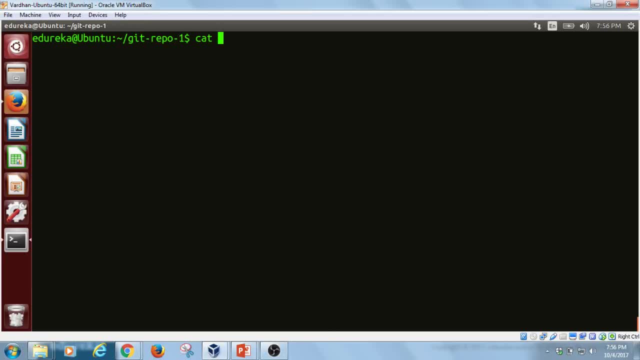 change you make to that code that can be saved like this and sent to get up in a similar fashion that I'm gonna show you now. okay, so now that I've added my code here, what I need to do next is I need to do a git add command. okay, so this would basically track all the changes that you do. 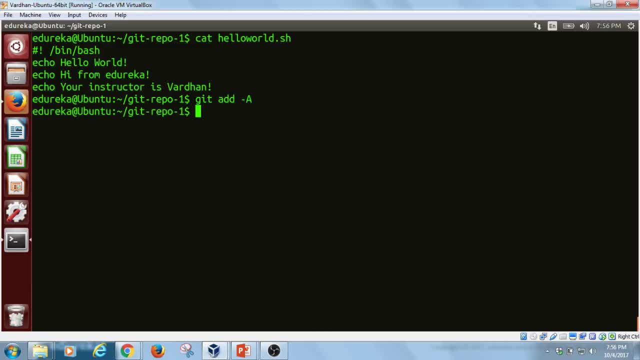 whatever you add, all that would be tracked with the help of the git add hyphen, a command, okay, and if you want to commit your changes, then the command for that is git commit with a M flag, which basically is to specify any comment. what is this comment for? so I can say that this is, this is the 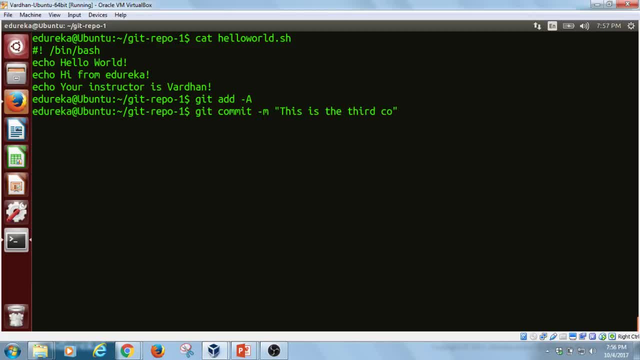 third line which I've added something like that: right, and I can say this is the build number three, or something like that, I can hit enter. so this is just the comment that would be associated with this git push of mine. okay, and to actually push your changes to your github and to get the changes there, there's this command. 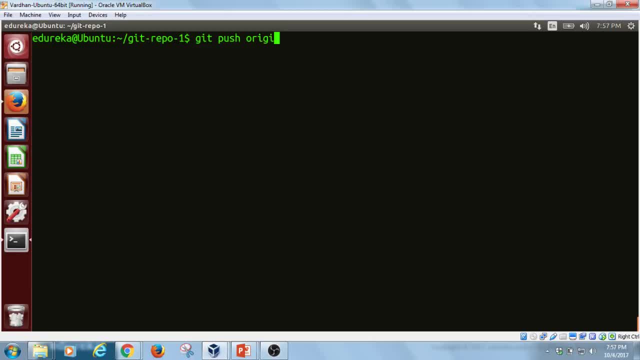 called git push origin master. okay, so this would push whatever changes you have locally. it would push that changes and then it would push the changes that you have locally and then it would push this to the github repository. so it will take a couple of minutes, so let's just wait till then. 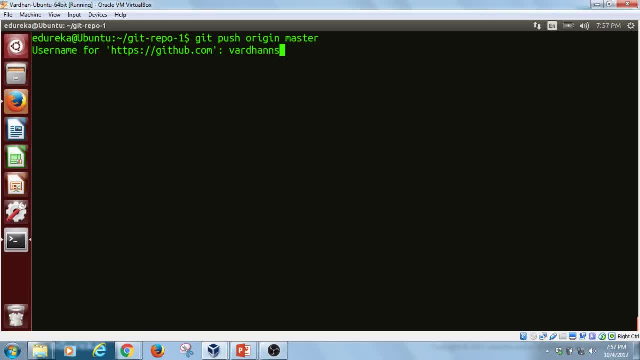 okay, the username is this and my password is this. okay, uh, maybe my password was incorrect, so let me just try hitting the command again. or maybe there's a problem at the github server, so let's not worry about that. it should be fine by just executing it a couple of times. 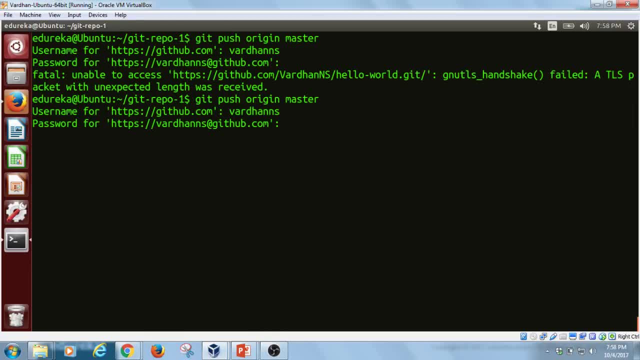 okay, there goes the username. okay, great, so counting my objects, compressing them, pushing them, done 100, so let's wait for the status. okay, great, so whatever i uh change, whatever changes i made, has been committed and sent to my github repository. okay, hello world dot git. so in a 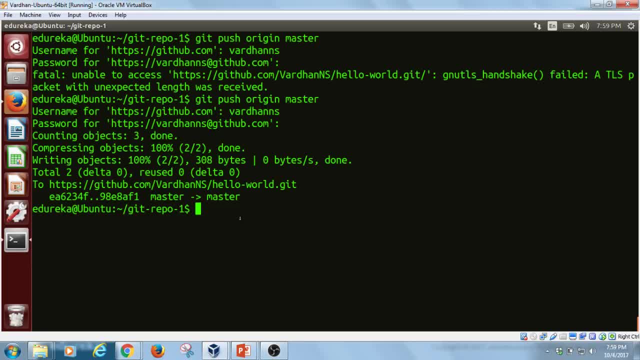 similar fashion. so developers will have a single repository for their, for their software application, okay, and in that private repository they can develop the application and keep making changes to it and then, through jenkins, they can deploy that code. now to verify if my github has the updated uh code, let me go back to jenka, let me go back to github and let me refresh this page. 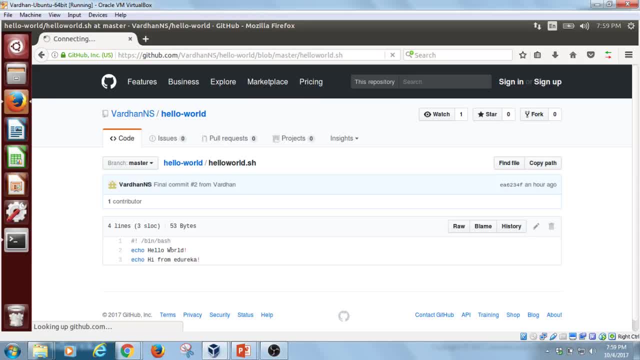 which displays what's there in hello world dot sh. a new line should appear over here, right, okay, seems like the internet is a little bit little slow, but anyways, that shouldn't be a problem. great, so the third line has also come in here. uh, so my github repository is: uh has the updated code. 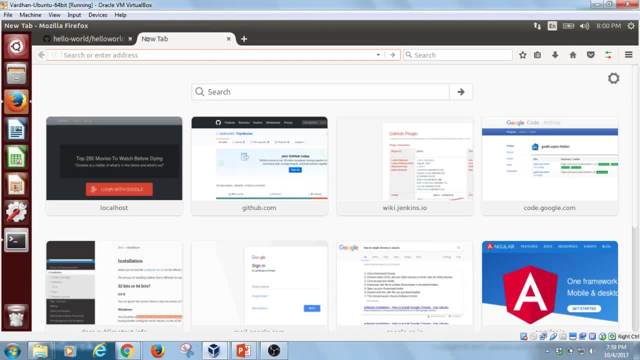 now it's all about jenkins. right now my jenkins is always by default hosted on port number 8080. okay, so if you do a local host, colon 8080, then you can access your jenkins web server and, uh, i don't think you people need to know anything. 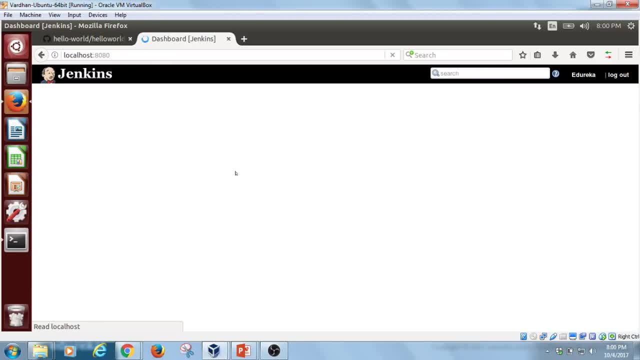 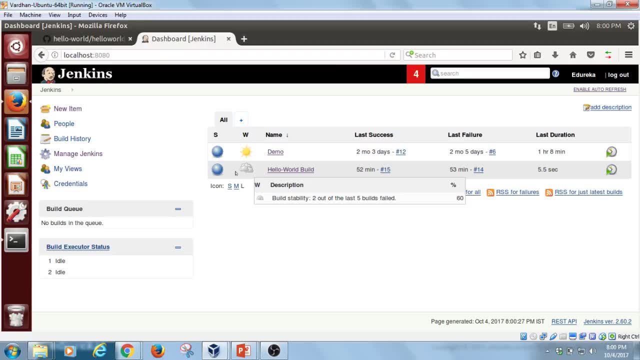 more than uh jenkins, being a web server which helps us pull code from git, and it helps us execute tests through testng and selenium. it helps us containerize applications with the help of docker. it helps us work with configuration management tools like puppet shift, ansible salt stack. 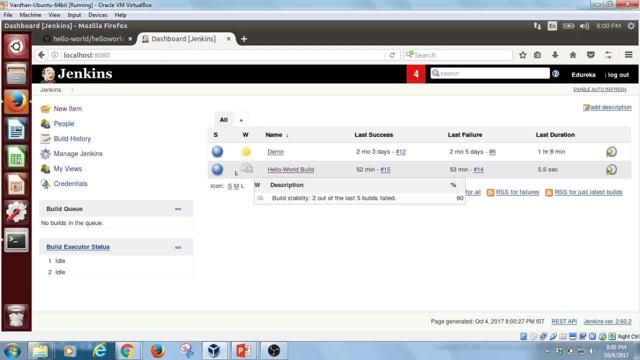 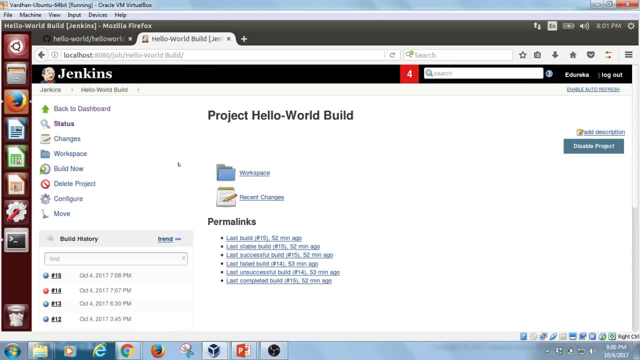 and, of course, it helps us in automating a lot of things. but uh, getting back to our session for today, the hello hello world build. so this was the project that i created, so let me just click on this and here, to save some time, i've already added my github repository here, so let me just 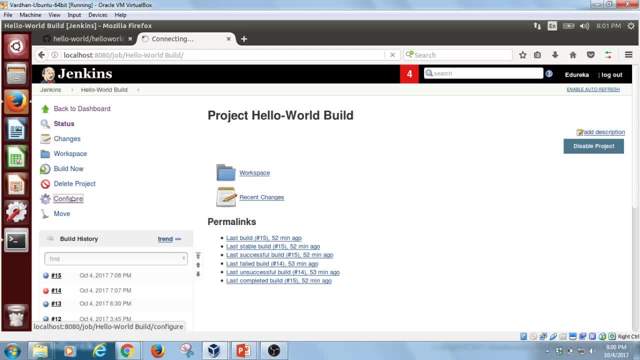 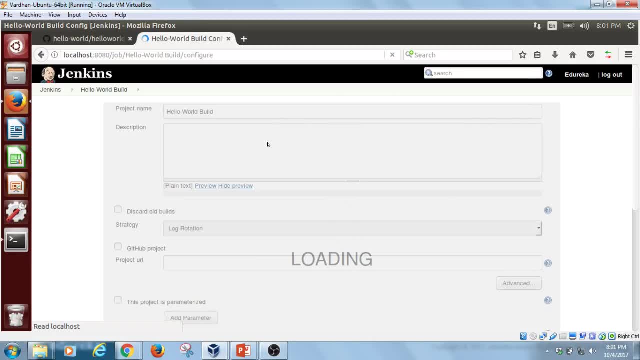 run through those changes, what i did. okay, to help you understand what i've done. so, under configure, if you go to configure you, you can make changes and you can add your project details. okay, okay, okay. so first of all, under general tab, you can add the project name. 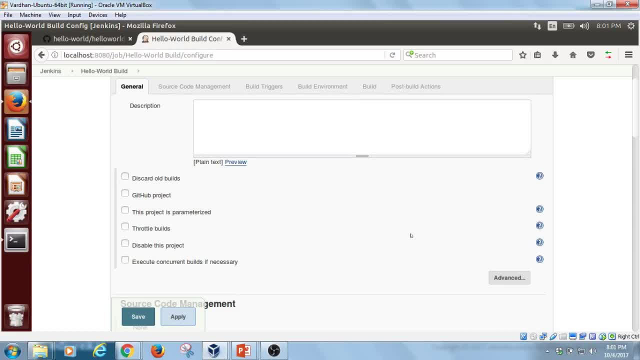 some description. if you want to- and, uh, in case you want to execute some comma, some file from your local system, then you can click on this advanced tab and say: use custom workspace space, okay, and then you can add the path over here. but since I'm executing this, 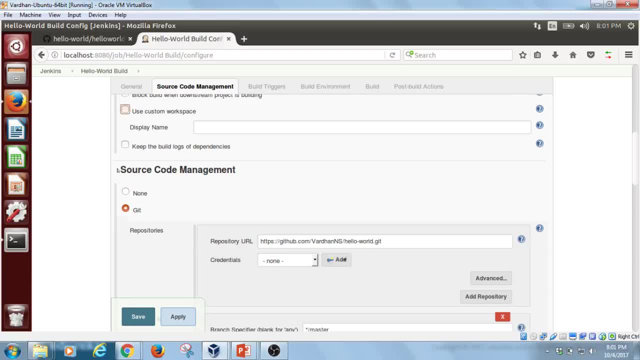 through github. I'm not gonna do that and it's gonna quickly go down. I'm gonna say source code management, I'm gonna say get a repository, and I'm- and I've specified the github URL. okay, slash hello world dot get. that's where this is present. my 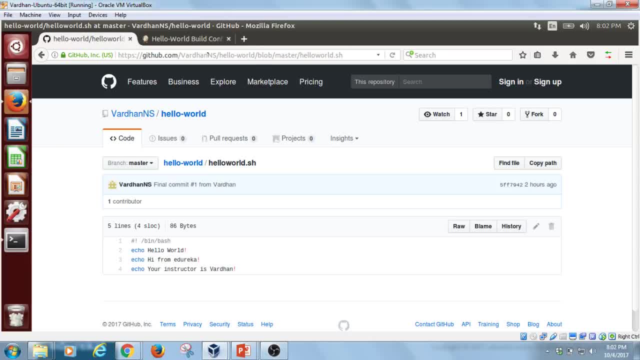 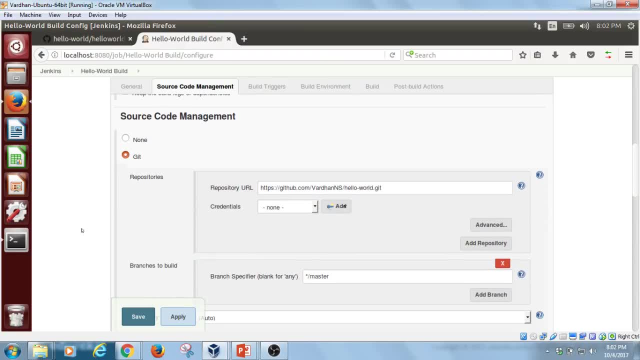 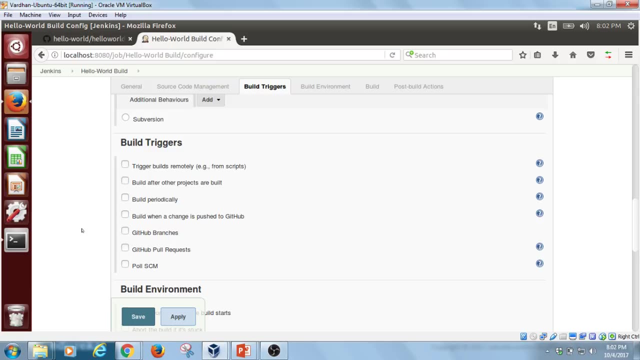 hello world. bash file is present under this repository, right? so that's what I have entered over here and you can just quickly go down and, under built triggers, you can control how we want Jenkins to execute. well, the actual concept of automation can be achieved over here. okay, if you want to, you know trigger. 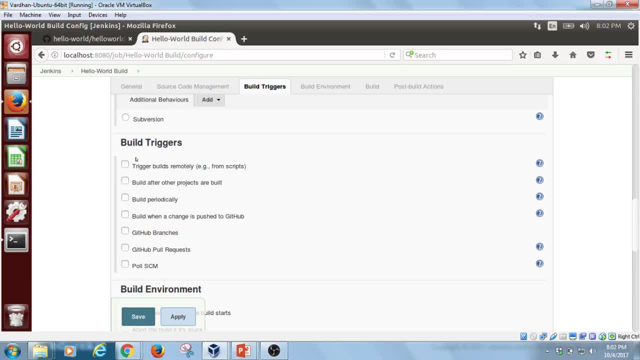 builds remotely. you can choose that option. if you want to, you know, build some trigger of this project after some of the projects, then you can do that too. if you want to build, build this particular, uh, if you want to build this particular job on a regular basis, on a periodic. 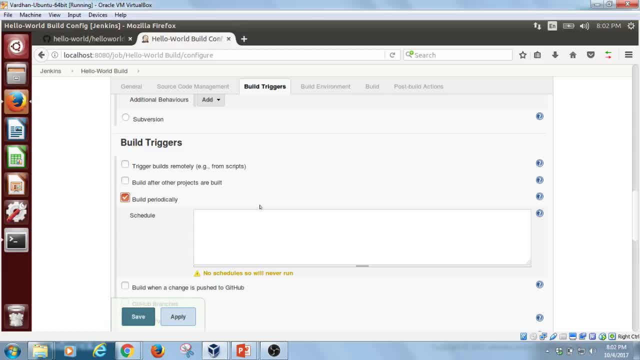 basis, then you can do that too. if you say build periodically, then you can in cron period, you can in cron format, you can specify uh once in how many hours or once in how many days you can you, you can execute this uh file. you can say that, or whenever there's some kind of change, that you push. 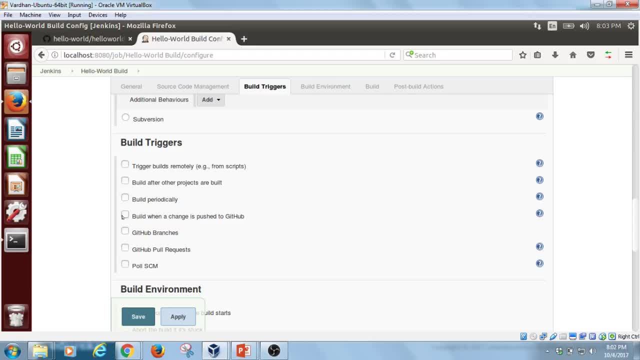 to get up at that times if you want to, if you want to get to execute, if you want to get sorry, if you want jenkins to build this job, you can choose that by checking on this and various other options you have. okay, so the automation concept is achieved over here. build triggers and then you have a. 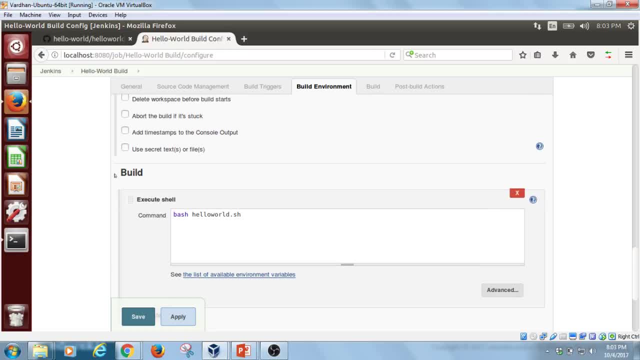 built environment, which we don't really need to worry about now, but the actual build. so here is where you specify what you want to execute. so i've given the, i've given the repository of my github account and, uh, over there there is this hello world dot sh file, right? so the same command which i executed. 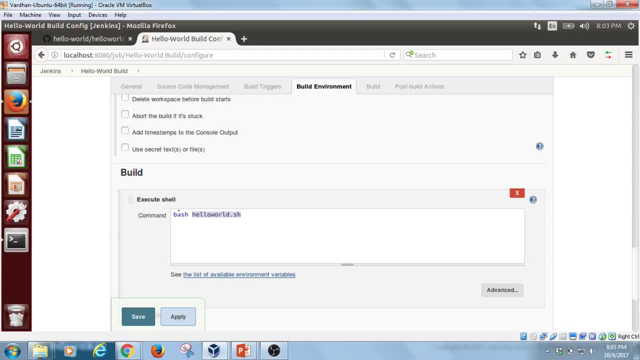 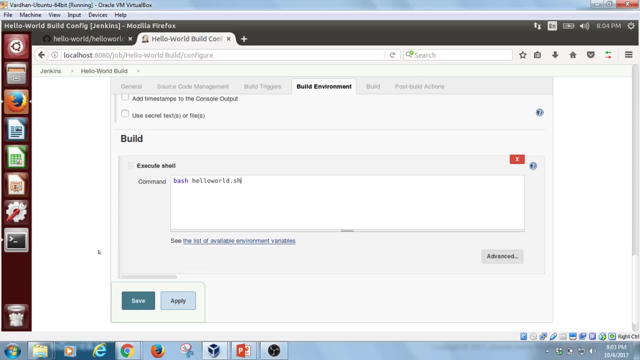 on my terminal i'm saying jenkins, to execute that same command over here. so in my shell i would be executing the bash command, and the file that i would execute with the bash command is the hello world dot sh. okay, it's as simple as that. so when i uh just build this job, then i would get the same. 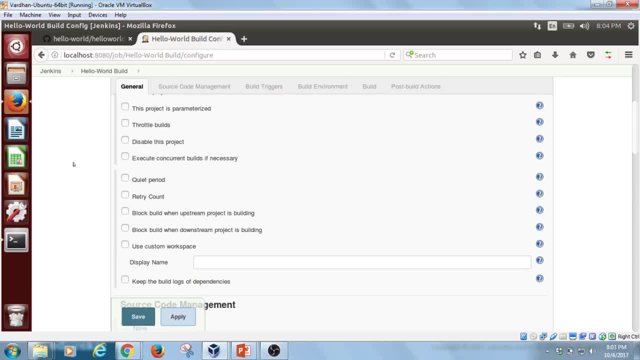 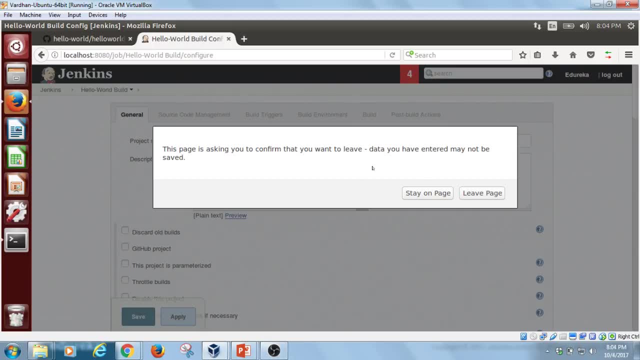 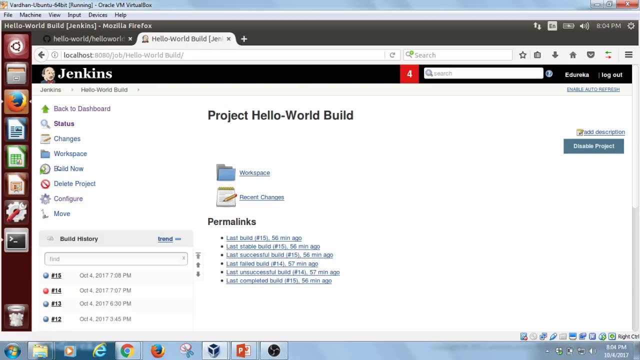 output i got on my terminal. okay, i would get a hello world. now let's see how you uh, let's see if that happens. so for that we need to go to build now. so i'll say i don't want to save any changes and uh, yeah, you can see build now option over here right above configure. so you 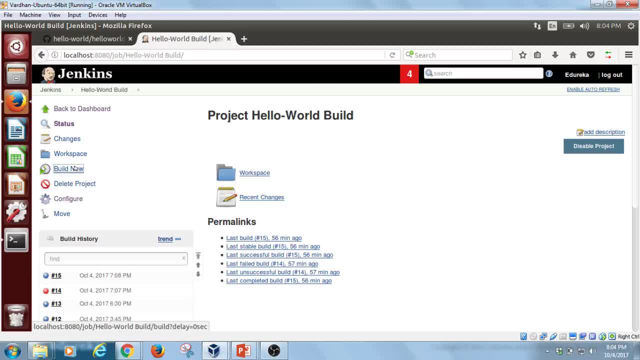 can click on build now and your, your job is would probably be getting built now, right away. so the build number 16 is uh scheduled and if you click on the drop down and if you go to console output, you will know what is the build number 16. and if you click on the drop down and if you go to console, 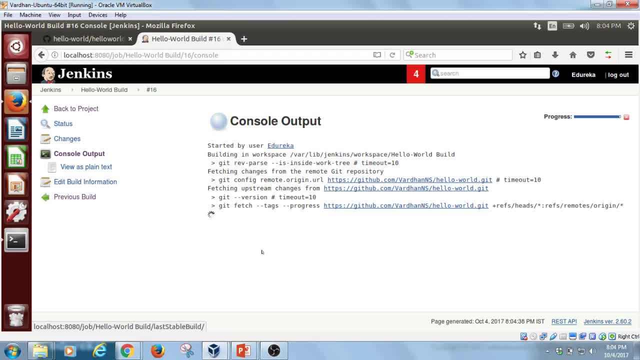 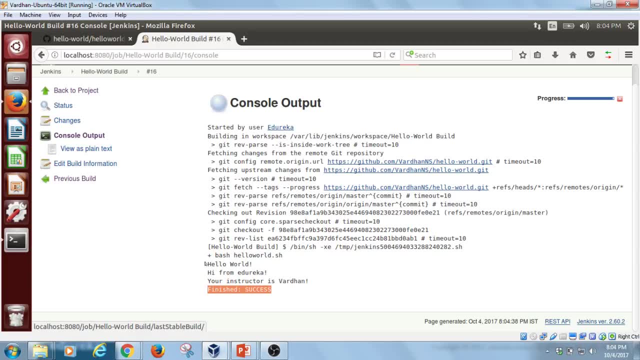 output. you will know what is the status. uh, is the uh built successful, is it not? and all these details you'll get so great it's a success. right, the finished state is a success. and the same three echo commands that i had specified in my bash file. they are executed here correct. so in a similar way. 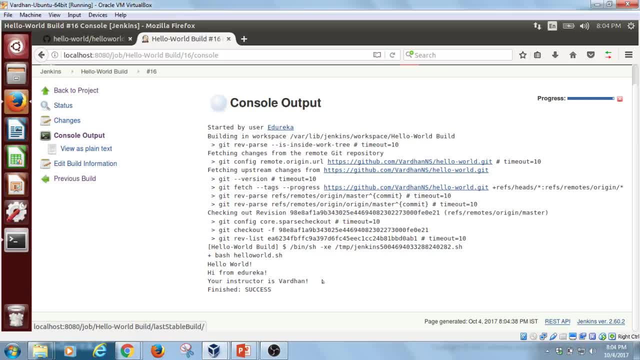 if there is any uh application that you have, if it's a java program or if it's a python program or if it's any kind of web servers that you're hosting. so in my previous session it was angular, which I, it was angular, and then one of the time I executed mean stack application. So these were. 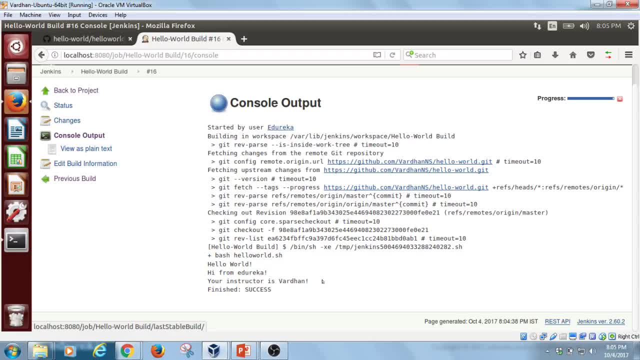 the things which I executed through Jenkins and Docker right. So similarly I've done it here, but raise very simple command. where I've you know is with a simple command, I've executed a bash file, But what you need to understand is this: is how Jenkins can be used in the industry. 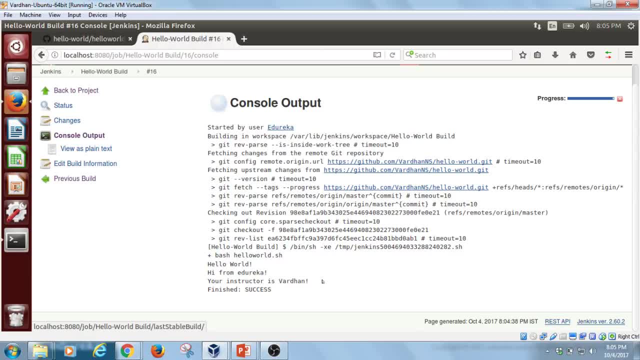 right, And this eliminates a lot of problems. There's a lot of scope for automation And there are a lot of benefits with this. So, yeah, that pretty much brings an end to my session here, So I can just wrap up my session by going back to my slides here. 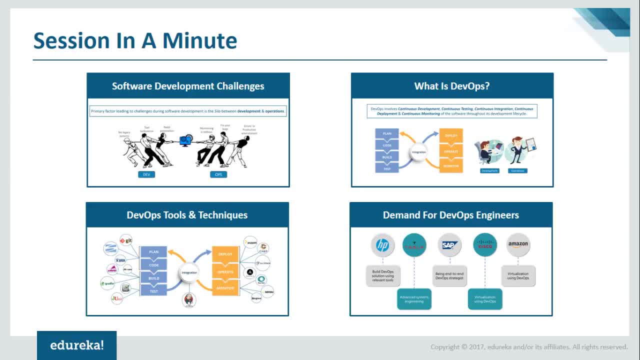 And guys do drop in your questions, I will take them in a couple of minutes, in a couple of minutes. sorry, And yeah, these are the topics that I covered. So I spoke about the software development challenges that are there, that used to exist. 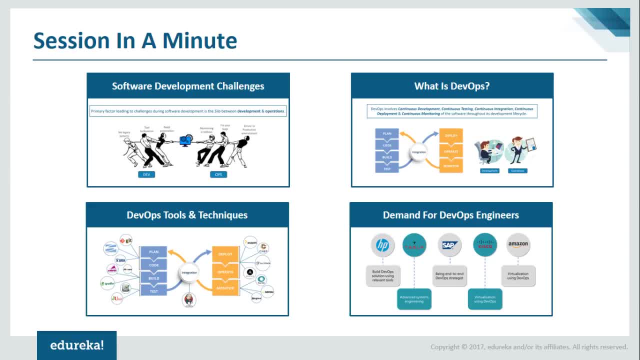 with the various models, And then I spoke about what is the role of a DevOps engineer And how the DevOps strategy, what are the phases involved over there, And then I told you what are the different DevOps tools and the different techniques to achieve automation. 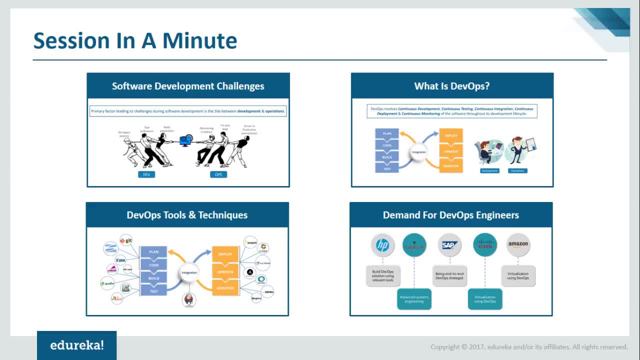 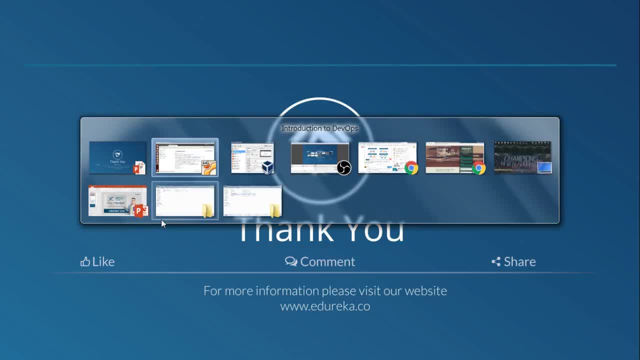 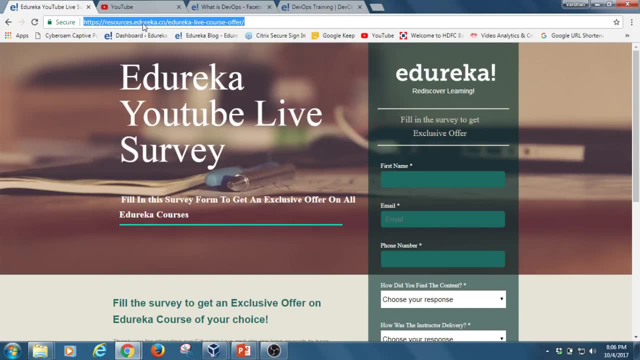 And then I finally spoke about the demand for DevOps engineers. So so, before I take up your questions, I want to just quickly show you this. I want to show you this survey form, And the link of this survey form is something that you would. 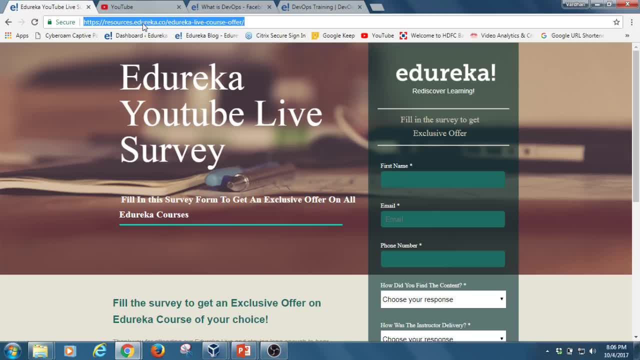 find in the comments below. So if you have any questions, feel free to ask me in the comments. And it's really essential and really important you fill this form if you want to avail exclusive discount on any Edureka course. Okay, and since you've been in session for so long, 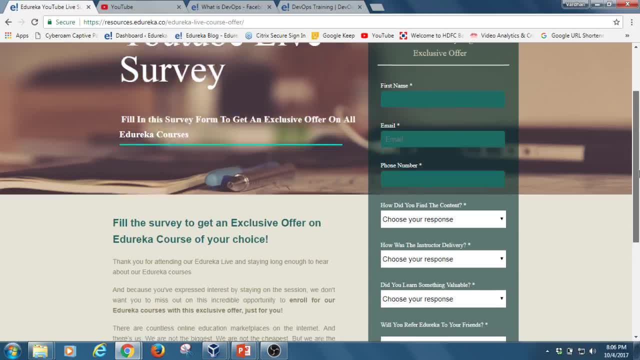 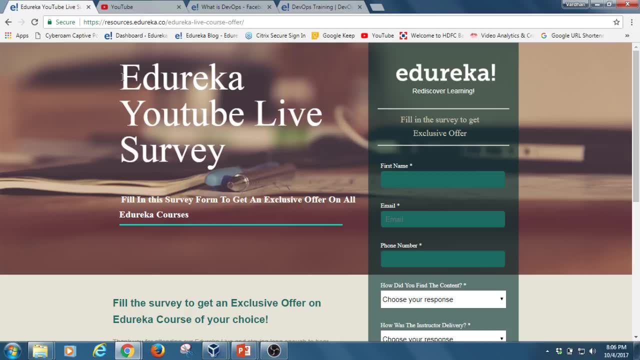 you're getting this link, So do take the small trouble of filling up these details. And yeah, so next time I know you're buying any course from Edureka, you can be rest assured that you're going to get a whooping discount on the course. So that was that. And then we have a YouTube playlist. 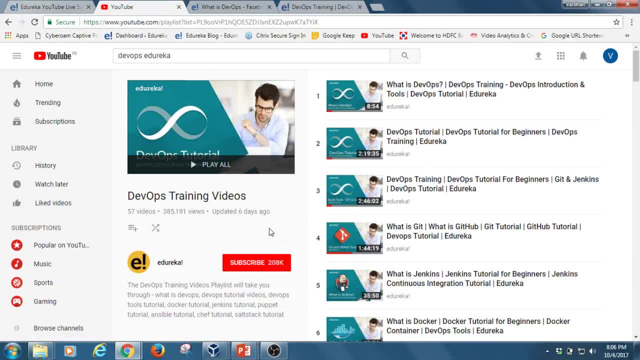 filled with the number of DevOps videos. you can check them out. you can like them, subscribe to these, to the, to our channel and follow our videos, like our, like them and share them. You can also check out our DevOps blogs. Okay, so we have a number of blogs here on each of the different 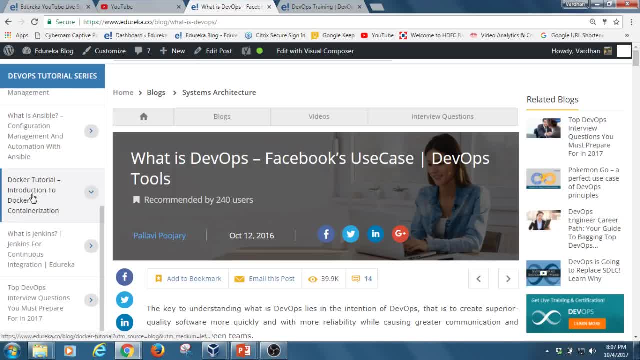 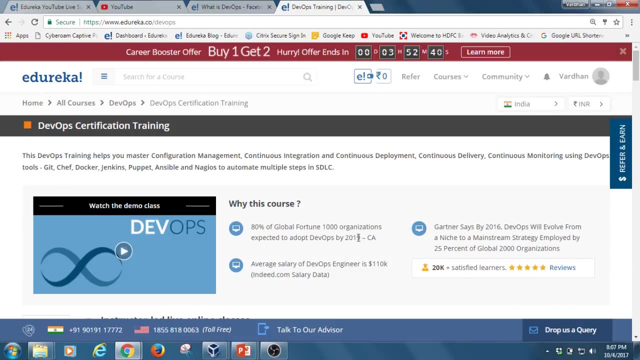 tools, on get puppet chef Ansible, on Docker Jenkins, And you also have an interview questions blog here. So if any one of you are interested and if you are aspiring to be a DevOps engineer, I would recommend you to go through this blog here. Okay, do that And finally you can. 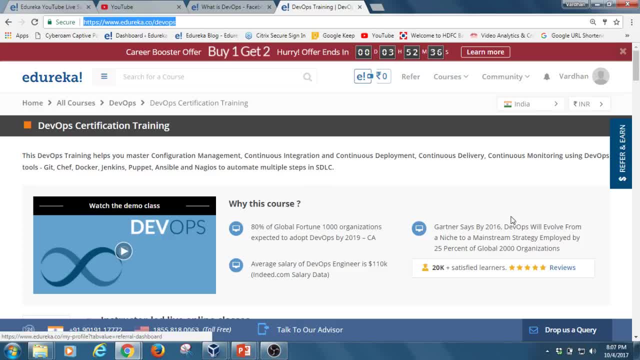 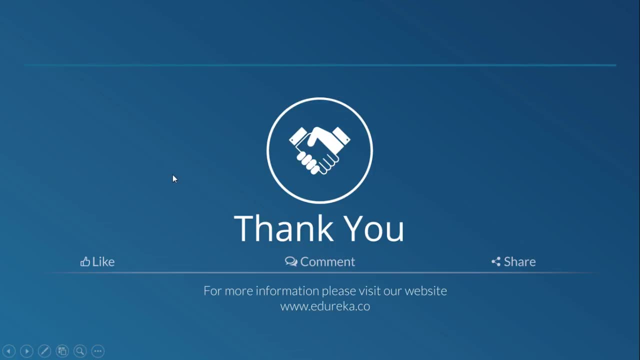 check out our DevOps course at this link, So you will find other details with our course with you know, with respect to the course details, the pricing and all these things over here. All right, So that's, that's the thing, guys. Now let me just see what kind of questions have been asked. So, 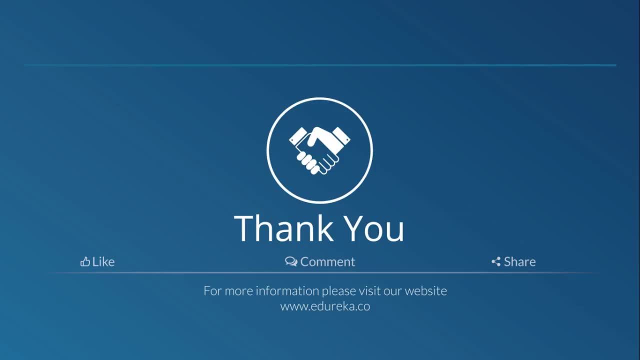 let's see. Yeah, there's a question here that says that clear on Jenkins. but there are multiple monitoring tools like SolarWinds, nagiaws, PRTG, BMC, etc. So why are we sticking only to nagiaws? 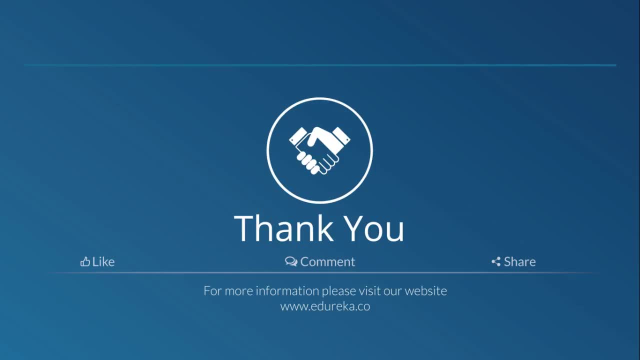 We are not just sticking to nagiaws. Nagiaws is actually my. it's the most comfortable tool. It's actually my most comfortable tool. okay, it's one of the best. and, uh, you can. you can implement the other tools also, so it's all up to. 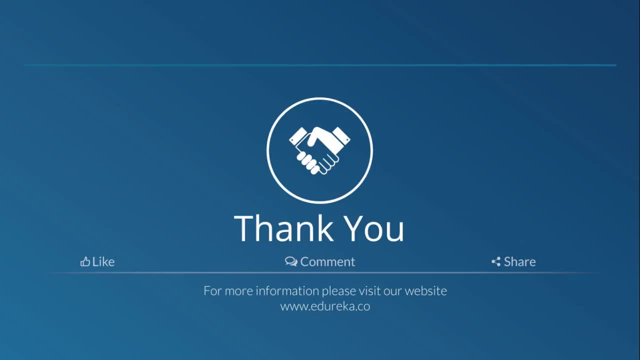 you and your requirements right, so all these may be good enough. so it's, if you feel any, uh, if you feel if it's important, you can execute and you can use them all right and uh, okay, okay. i have another question here, which is when will i conduct a live azure uh admin class? uh, sure, uh, sri will. 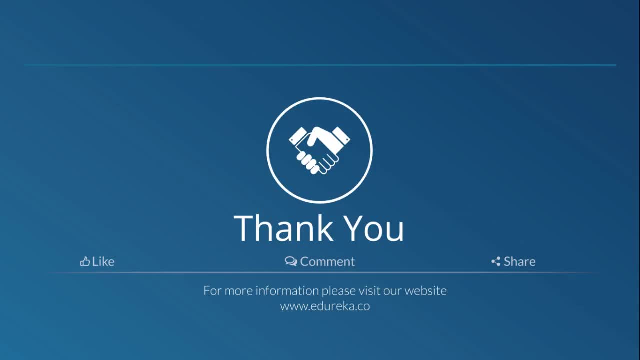 have it uh very soon. thanks for your uh you know question. so we would i would uh send this feedback to my team and we would have one very soon. we have another good instructor for that and uh, we'll make sure that that happens. and there's another question: jenkins is used for development. nagios is used for uh monitoring. well,